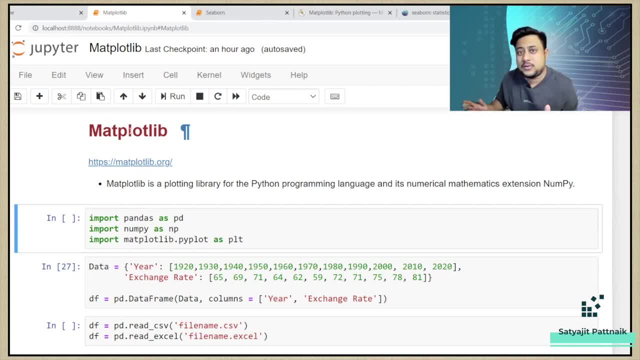 and again. So let's get started. This is an ocean, and covering an ocean in just 10 minutes, 15 minutes, is very difficult, but definitely this video will be a kickstarter in case you are new to this, In case you are new to: 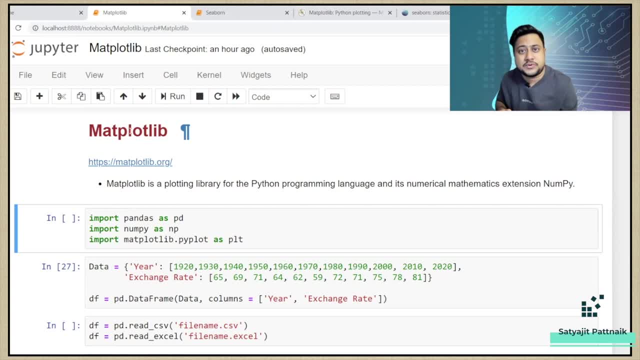 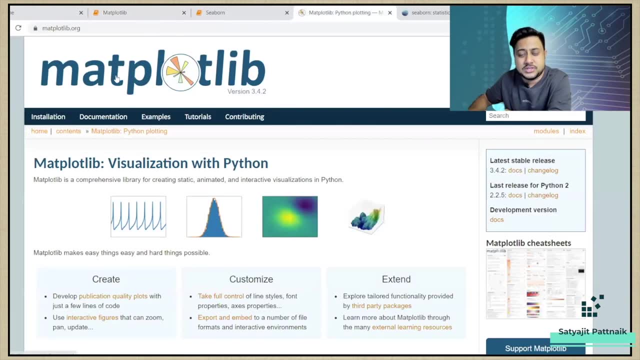 data science. new to data analytics? definitely, this video is for you, So let's quickly get started. Matplotlib- anything and everything is. you can find it over their official website, which is matplotliborg. You can see there are many visualizations with python. Matplotlib is a. 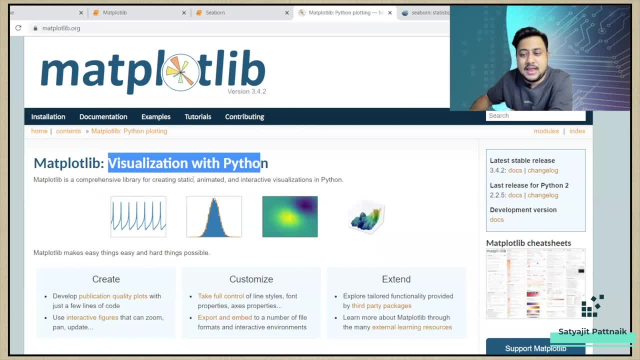 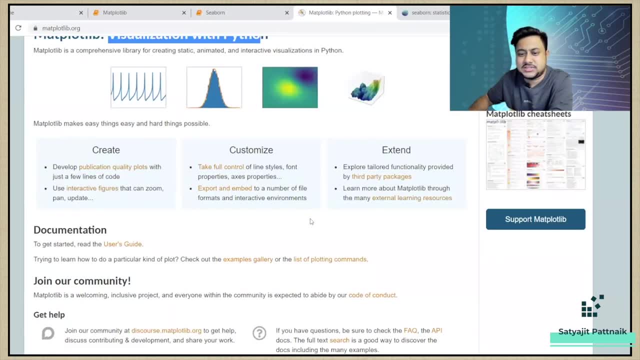 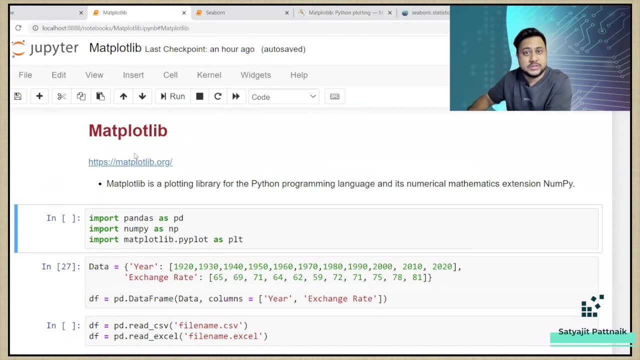 comprehensive library for creating static, animated and interactive visualizations in python. Many things are there: create, customize, extend- So you can just go through this blog. I will leave this blog description, blog link in the description below and we'll talk about this jupyter notebook. 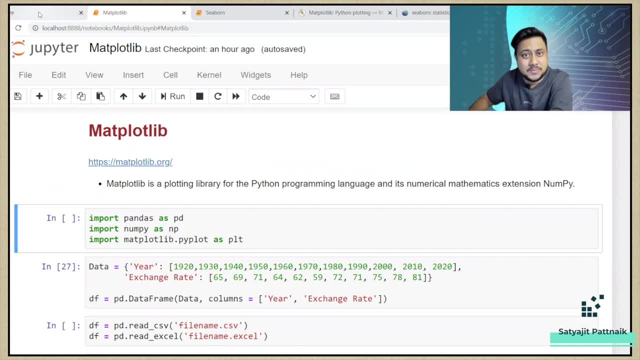 which we have already created, I think pandas and numpy. you already have gotten that links. I shall be sharing matplotlib and seaborn with you. So matplotlib is a plotting library, It's a for python programming language and its numerical mathematical extension, numpy. So here we are going. 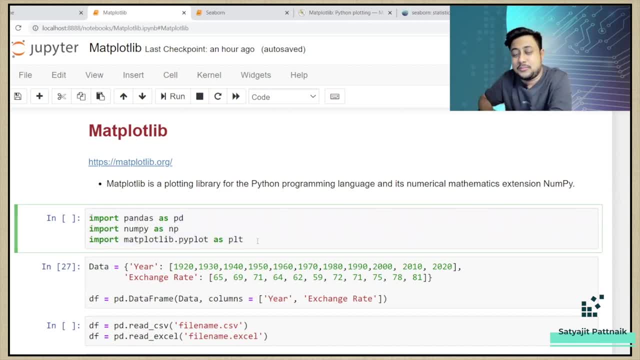 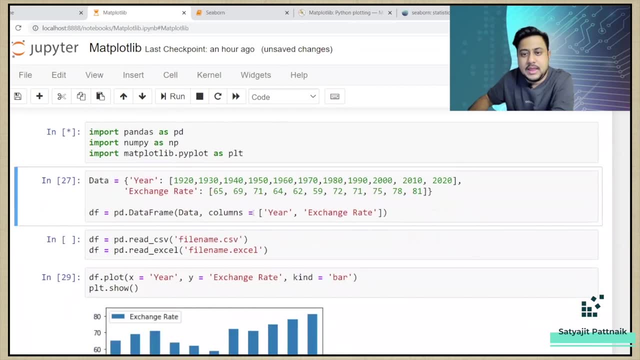 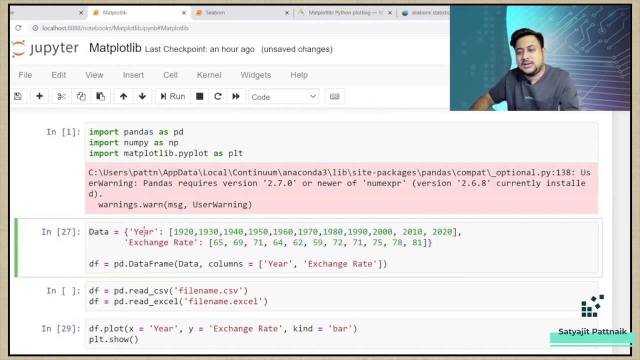 to import all these three trio, the three mosquitoes. So we'll import pandas, numpy and matplotlib. So here we go, In the next step. what we have done is I have simply created a dictionary. You can see, I have a year and then I have exchange rates right. So we have created this. 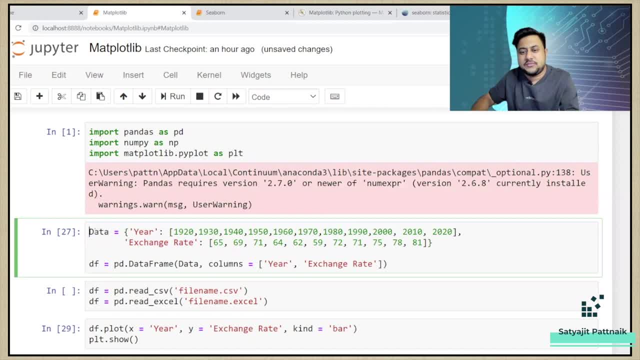 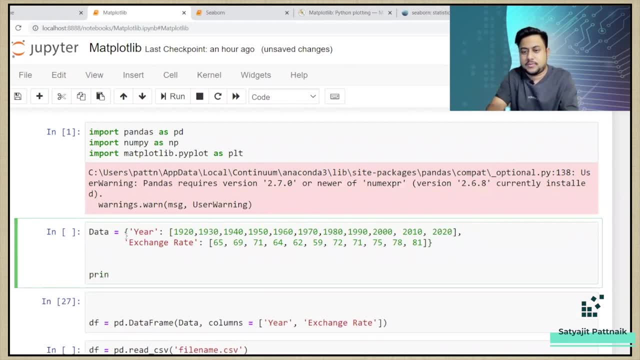 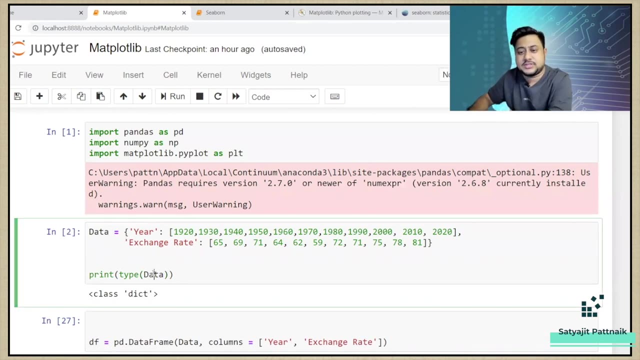 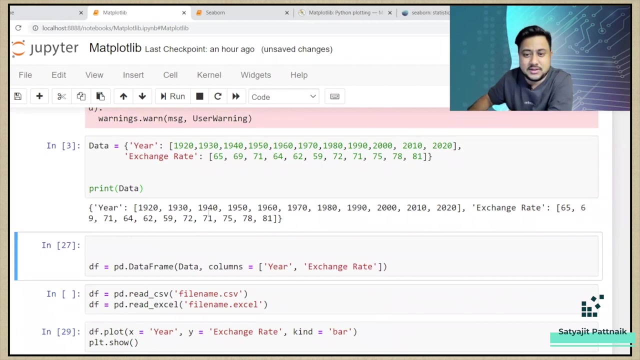 and then we are converting this data. You can see if I just run this. You can see this is how my dictionary looks like, my data, and if I just have to print it, of course we will be able to see the entire records here. and then we have the exchange rates right. So in my 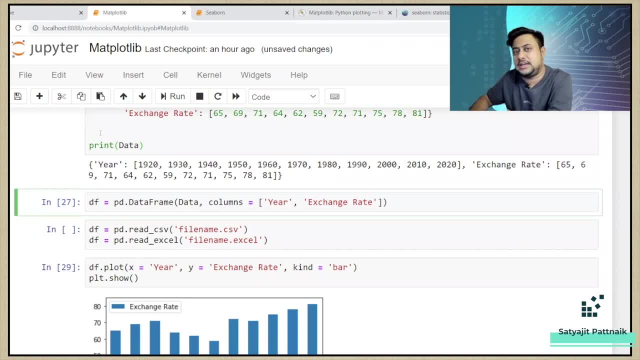 next step. what I am doing is I'm simply calling the pddataFrame. That means any type of object. if I want to convert it into data frames, then I'll have to use pddataFrame. In case you are reading a file, we know that it's going. 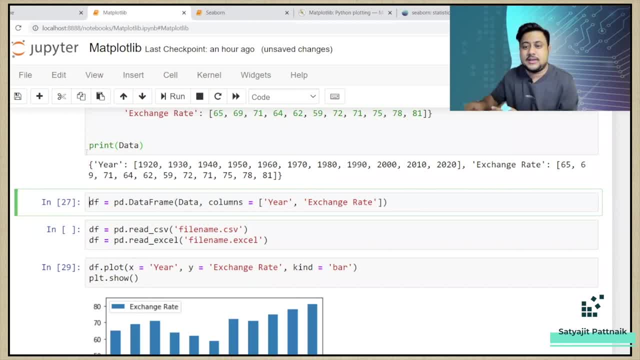 to be: return underscore csb and return underscore excel, right. So here we have converted a data into data frames. Here I'm passing the data, which is data, and then I am telling that my columns are going to be here and exchanged rate. So if I just run this, this is how my df looks like: dfhead. 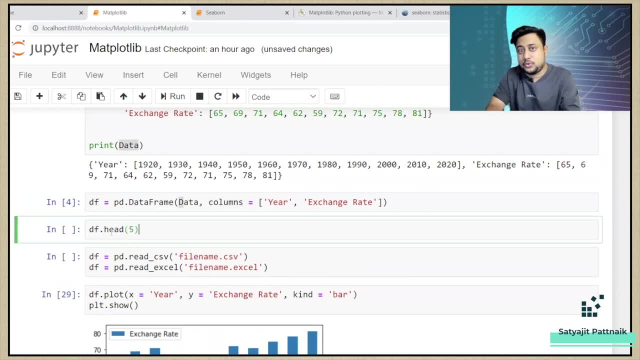 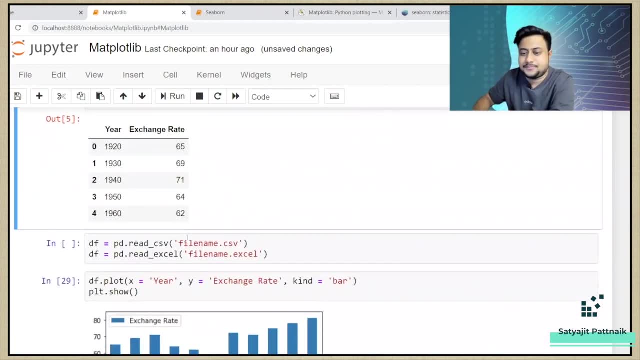 is the current index. In order to work with this, set writeiz and say, hey, I am not going to enter data. df looks like df dot head. i hope you know about head function. we have already learned in pandas, so this is how my data frame looks like now. of course, this is just an example to show you how. 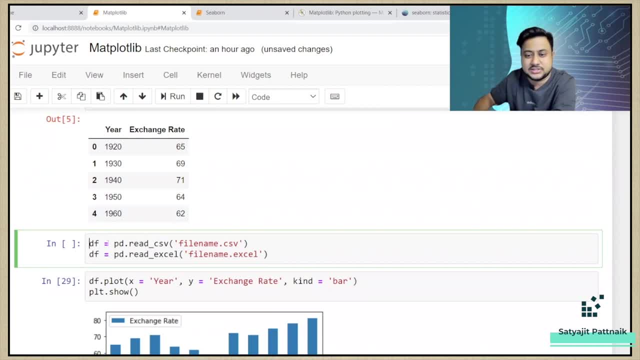 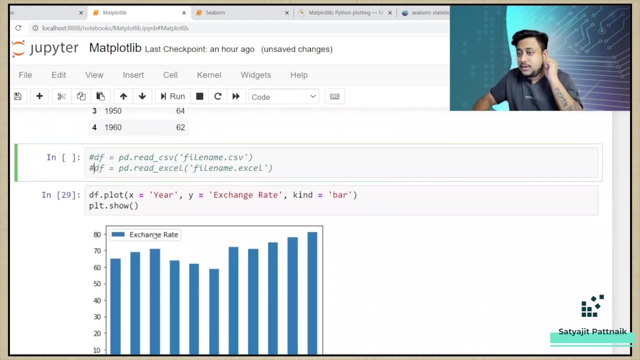 to read a file which is a csv format or excel sheets, right? i'm just ignoring this part. i don't want to run this, so i'll just comment it out and then i'm going to plot a simple bar chart. so here i'm calling pandas, data frame dot plot. but this code is not enough, right? so if i just 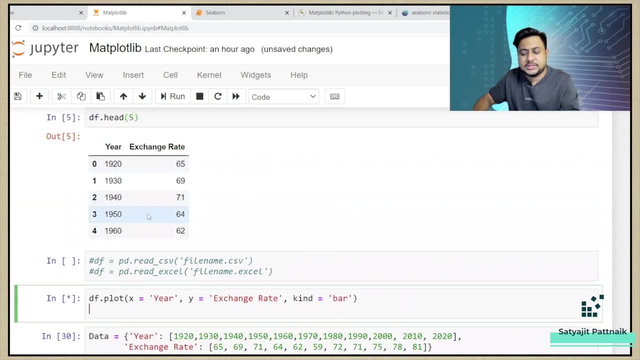 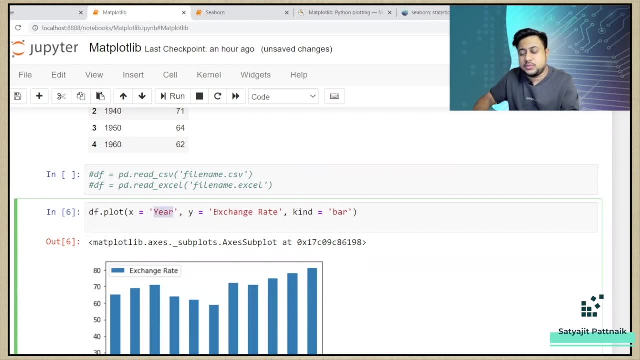 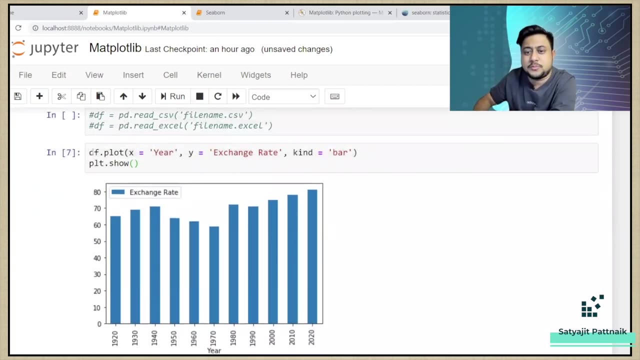 run this. this code will not be enough, let it. let it finish. df dot plot. i'm passing my x equals to year and my y equals to exchange rate. so we can. we can plot it using plt dot show or else without that. also, by default, it understands that if we are calling the plot function. 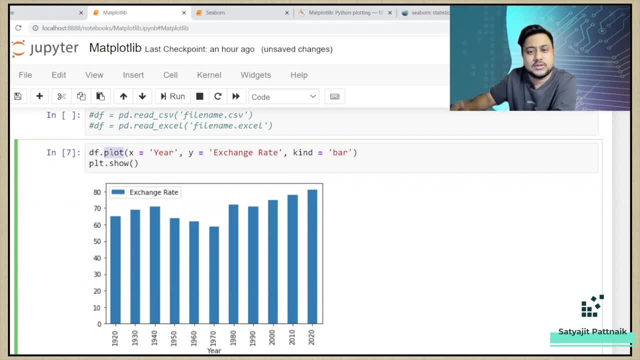 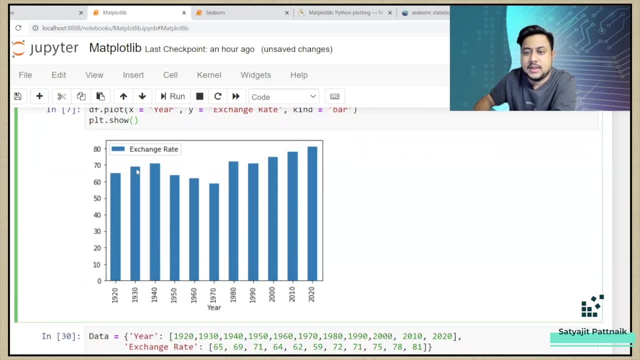 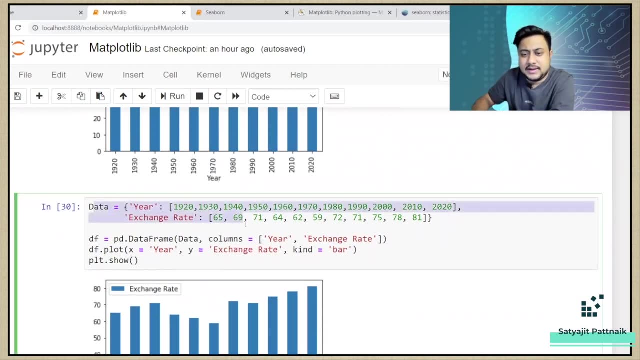 then it has to plot it using matplotlib. so that's how the dependencies has been created. so here i am passing my kind. equals to bar. this is a bar graph. okay, exchange rate and all those things, and then same piece of code. i'm again calling my data. so this is the same piece of. 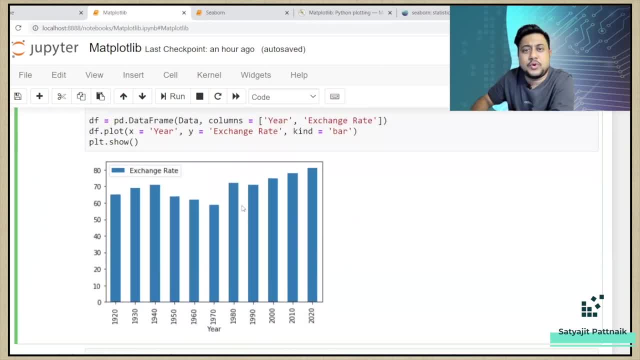 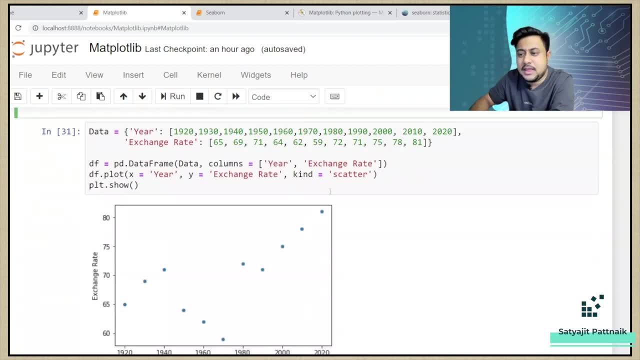 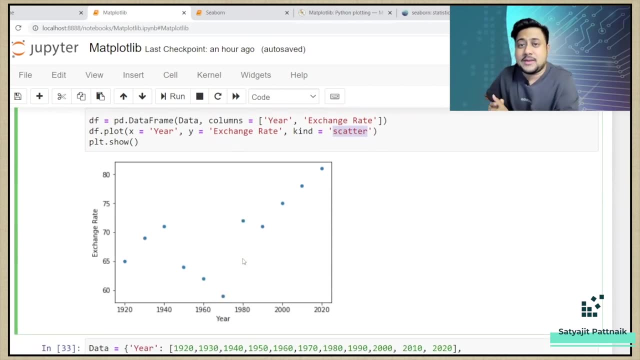 code. okay. so here, if i have to call a scatter plot, same piece of code, exact piece of code. but here, instead of the kind equals to bar, i'm just changing it to scatter. that means i can see the scatter plots. scatter plots are mostly used to analyze numerical data. let's say you have two numerical data: age versus area, or else numerical. 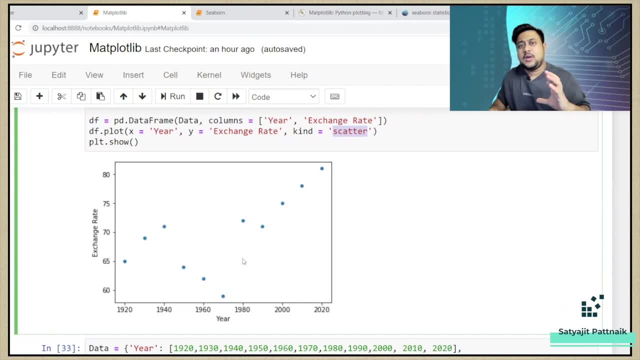 data one versus numerical data two. you want to see whether there is a linear relationship or not. you can probably print a scatter plot. there are some plots called as pair plot, which is basically, if you have 10 numbers, you will be able to see 10 cross 10 metrics and you will see diagonals will be the 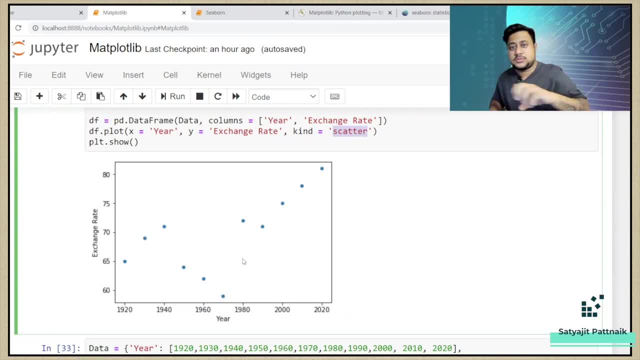 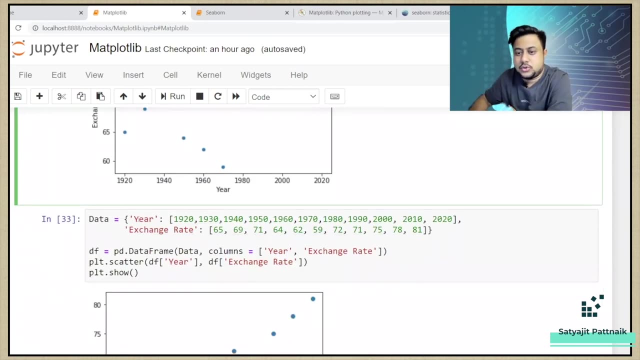 bar distribution, but the other parts will be a scatter plots within your variable one versus variable one, variable one versus variable two, variable one versus variable three. so all these graphs will be your scatter plots. we'll talk about pair plots as well, so majorly scatter plots are. 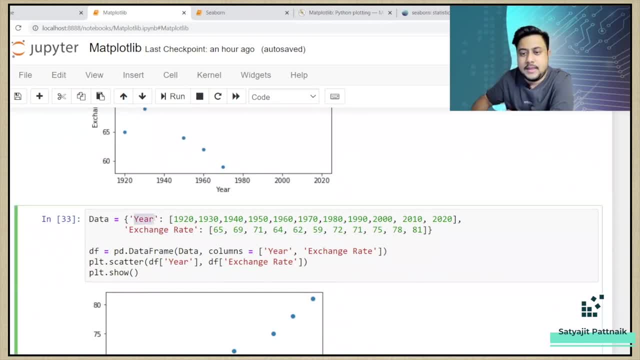 used for analyzing numerical data. okay, now, of course, i will give you ningún random number. but if you want to use even square number, then then do this 여기까지. you just need to first do it until you know the toward and between. but if you want to do what you don't know what you are analyzingWhy shall you do and answer the question: do you mean by zehn versus ten and what will be the jednak size? so that means we have these three lines and says: 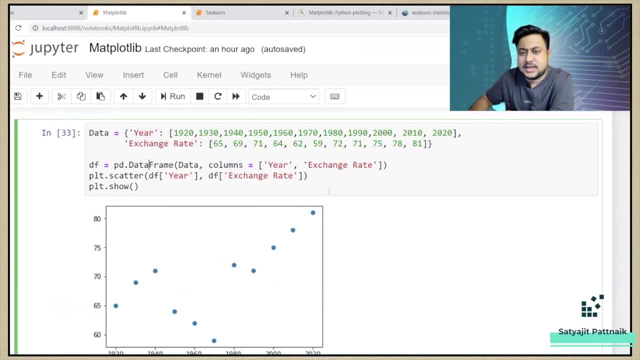 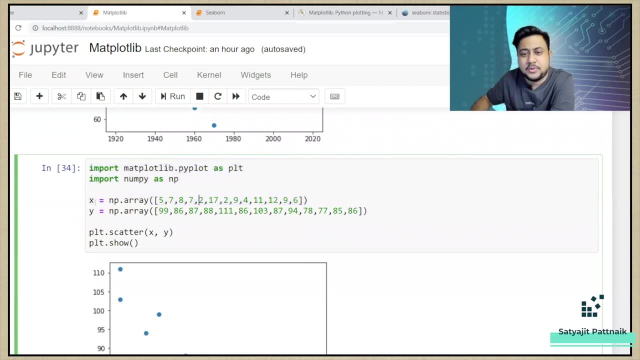 then it's simple, it's the same thing. i'm just calling the scatter plots. and here our next topic is, again, it's a scatter plot, a different way of creating a scatter plot. so here i have created a numpy array, my x and my y, and i'm just calling plt, dot, scatter, plt, dot show. okay, that's. 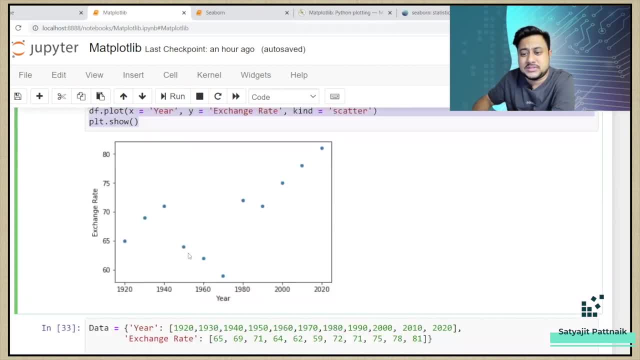 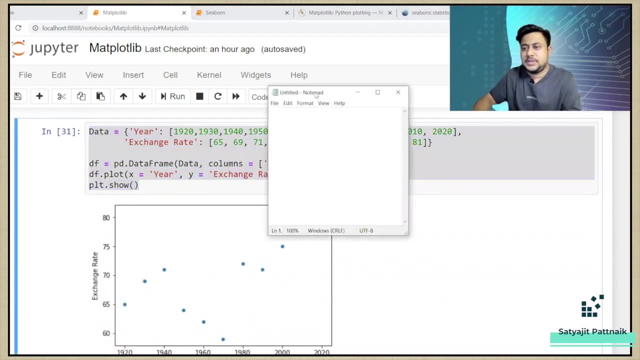 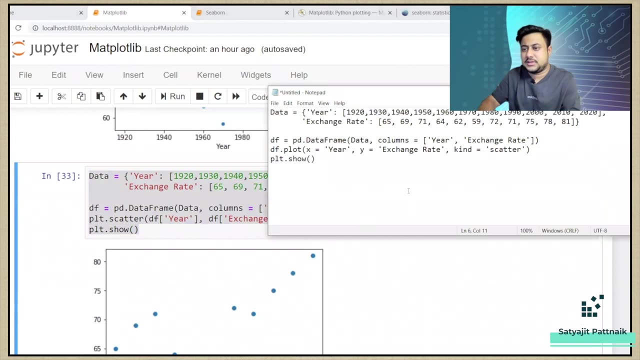 what i remember right now. i was just thinking: what is the difference between this and this? because the graph is almost same, you can see. i will just copy this code and i will paste it in notepad. and i will copy this code and i will paste it in notepad. of course, the first data. 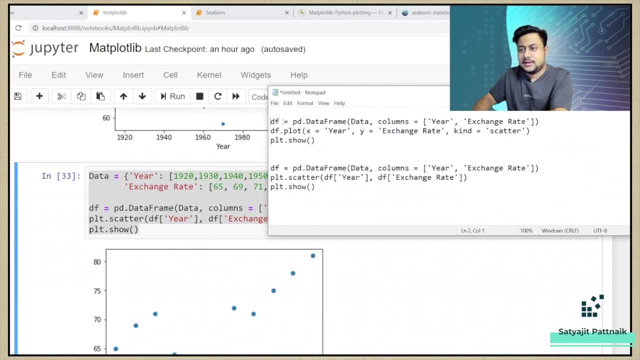 thing is common, so i'm just removing it again. the df equals to pandas. data frame thing is also common. you can see. the first part is: i'm calling pandas dot plot. i'm asking: kind equals to scatter. that's how you can create the plot using pandas library in matplotlib. 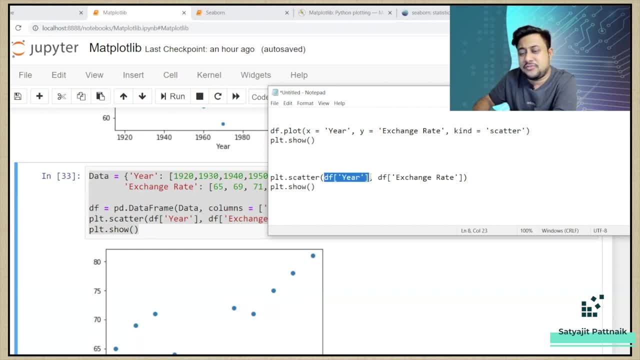 you have to call plt dot scatter. you have to call your df of ear and df of exchange rate. that means this is your x and this is your y. so this is how the formula looks like. this is how the base code looks like: x and y. okay, instead of that, i'm passing here. 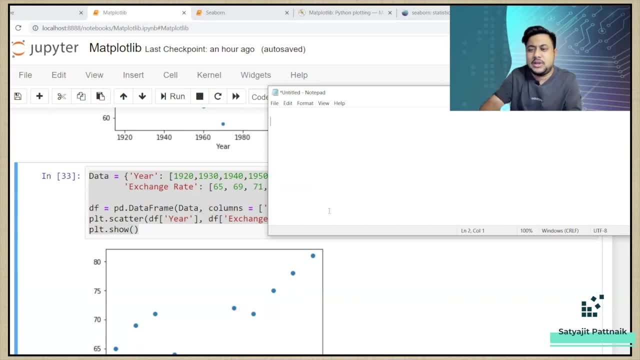 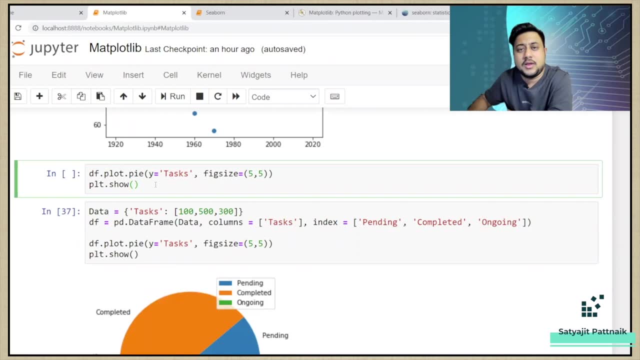 and i'm passing my exchange rate. so any of these techniques will give you a scatter plot. moving on to the next topic, which is going to be pie chart, where do we use pie chart? very easy, when we are having something based on 100 percentage, right, what were the total? 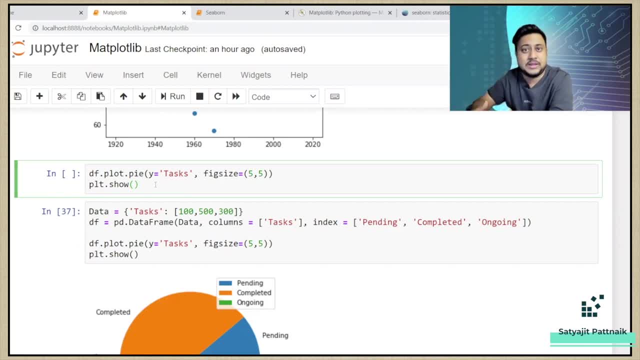 percentage distribution of males and females, or total percentage distribution of people who are taking mathematics and biology as their first elective. so all these things which you have to compute based on 100 limit, then probably pie chart is one of the suggested answers. so how to create a 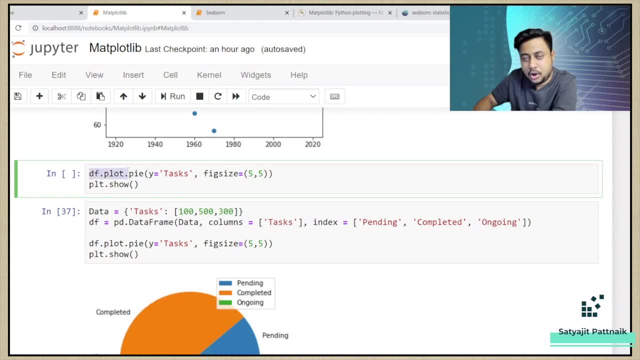 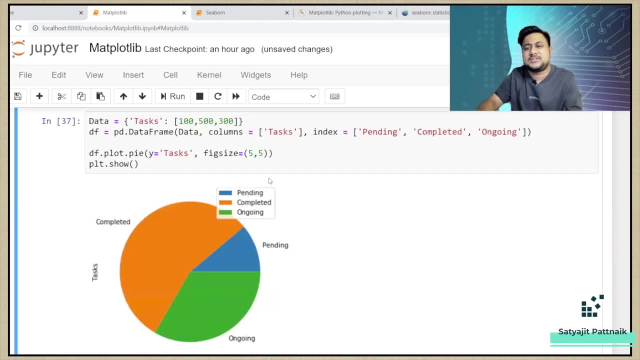 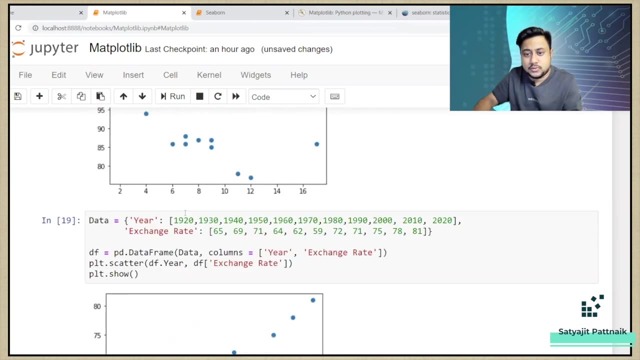 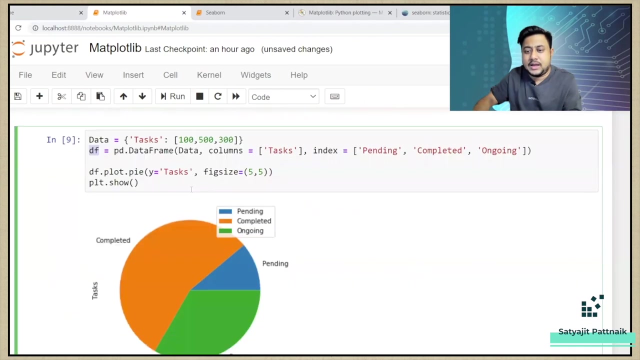 dam matplot divide pie chart with this, our equal Caion, and i'm going to say the one i'm putting as the die, valence and my difference is zero, because we have to divide this thing by 0.. мор and instead of another die for all ages. we're going to put it here, so make sure you get the and right. is shown me on the right side in the equation. so here's ourbia pad from five years ago, right, and then with that we have our difference in decision type, which is equal to X. now go running a. but i'm passing by piplot df dataframeplotpi. Y equals to tasks. here i'm just passing my figure size. if you just don't do it, that's okay. okay, so well, Y equals to tasks, so okay, tasks is not defined, so i'll have to create this. and then i have to pass df of taskslem, bigger of tasks. so this has to be a code which has to be run by what you're getting. 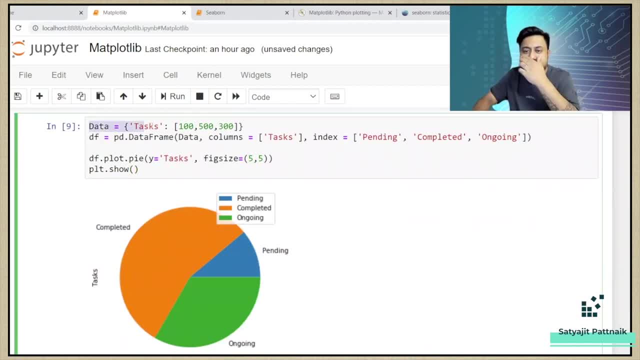 run after that one. so my mistake. so here i have created a data which is tasks 100, 500, 300. here i have converted the data to data frame. of course you are. if you are having a file, just read it and then you can just simply call this function in your y. you have to just call the tasks simple. 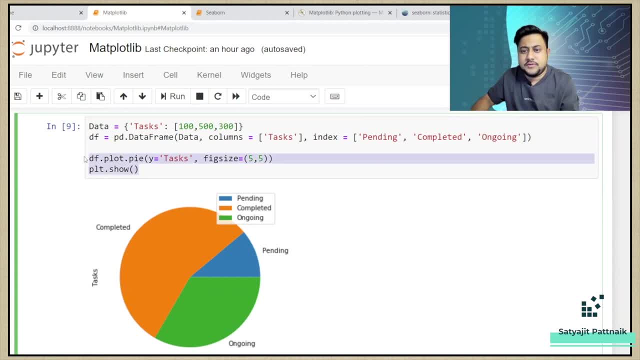 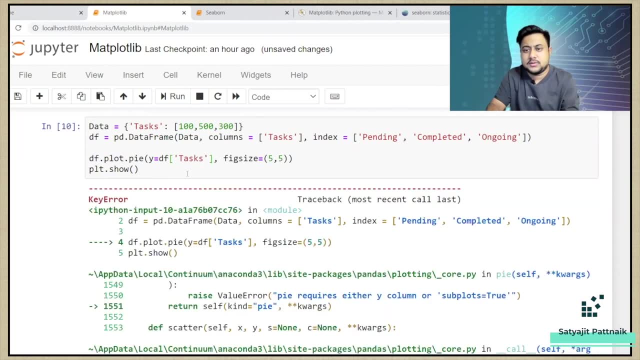 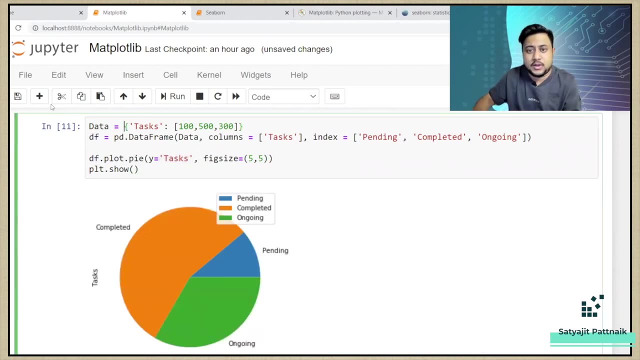 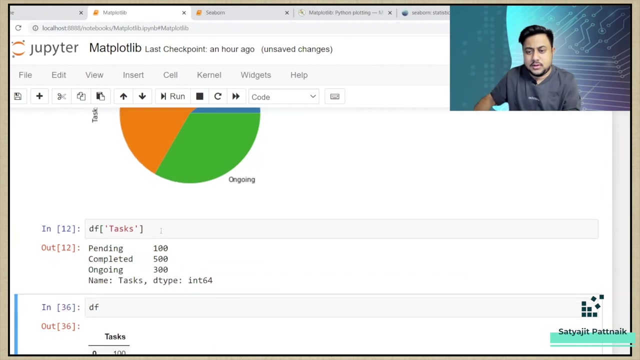 right. so here, instead of this, you can also do: y is equals to df of tasks. i think it should work. okay, so let's say what why it didn't work. let's see, we will see. okay, okay, okay, okay. so data frame dot tasks is basically giving me. so, because of the 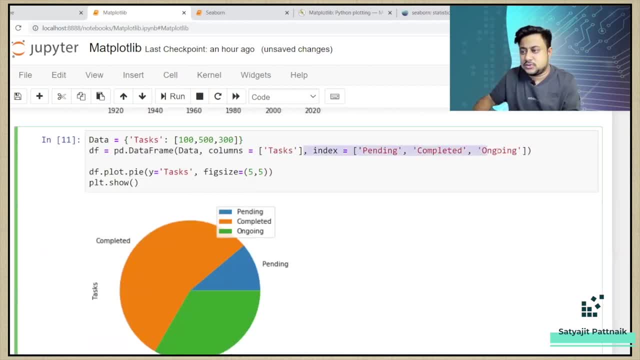 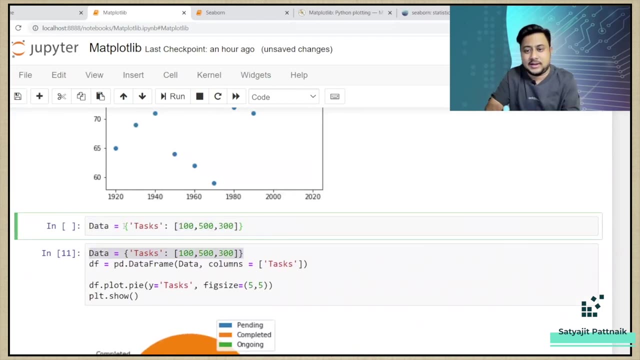 indexes. it is providing me this thing, so let me just remove it once. so if you don't provide the indexes, it basically takes the default index. right now. let's run this program one by one, then we'll be able to understand. so here i'm creating my data. right, if i have to print data, 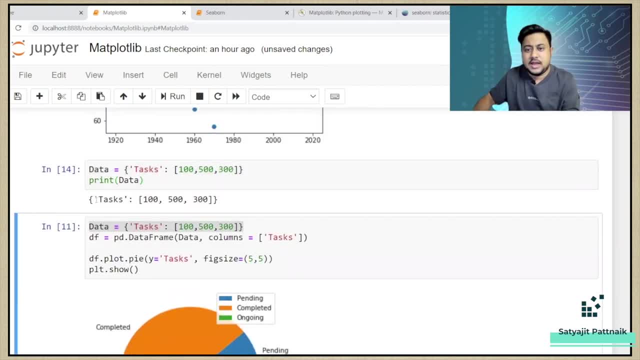 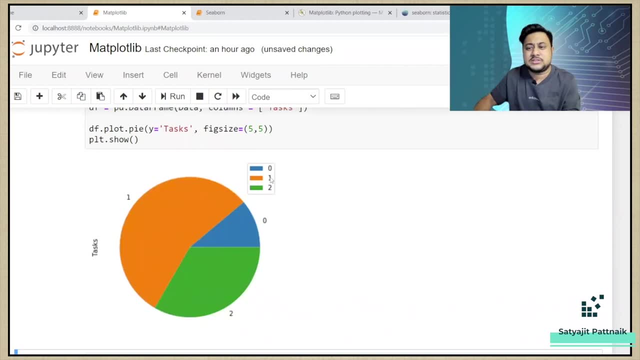 print of data. this is how my data looks like. i have tasks and i have these values. so if i'm running this code, of course i will get the list of the tasks and i will be able to get the data labels as zero one two, because this is how my indexes are. my indexes are, by default, zero one two. 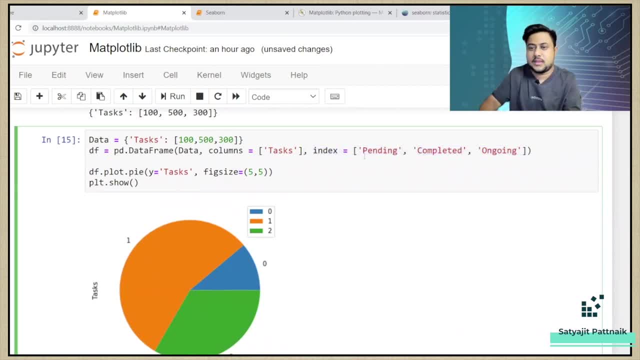 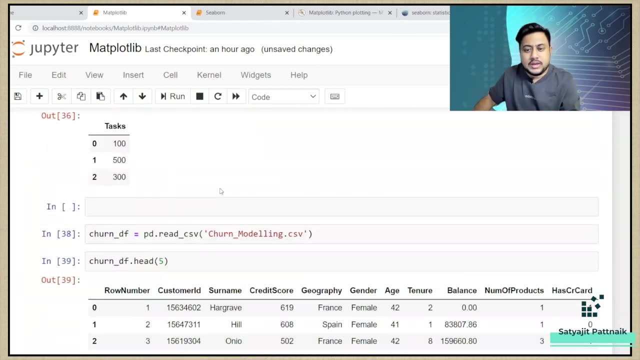 if you want to provide indexes, you can provide like this: okay, so here i'm just providing y equals to: okay, so why this y equals to df of tasks is not running because we are using the pandas dot plot dot pi. okay, so let's see, i think we also have matplotlib plot pi, as i told you, i have. 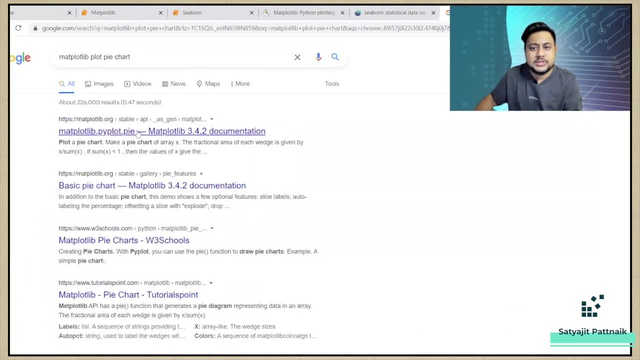 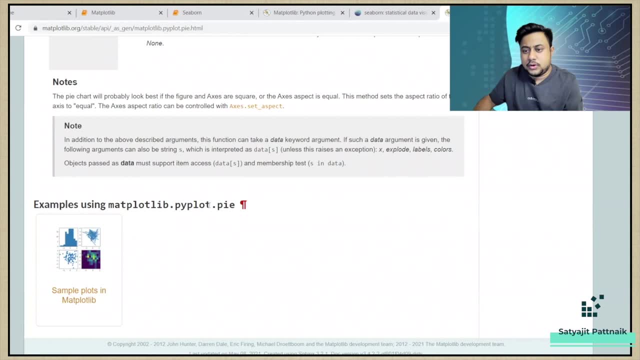 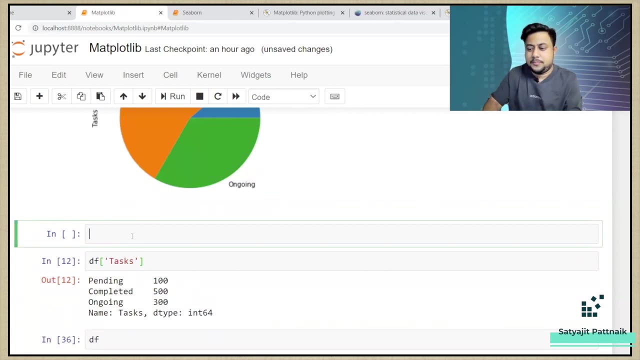 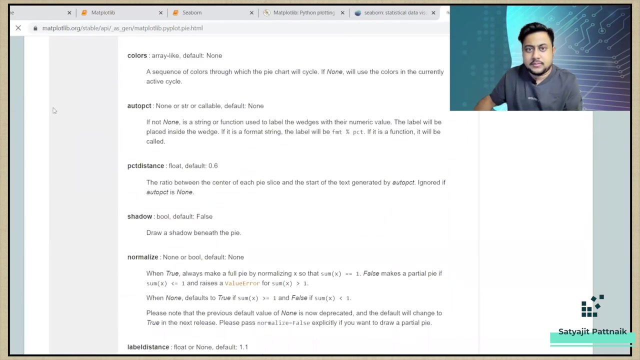 just created some charts. of course, there are whole bunch of things which can be done. okay, let's just quickly do that and i think it's really good- plotpi. i think it should work. let's do this pltpi and what- how to use it pltpi? let's just take some examples. 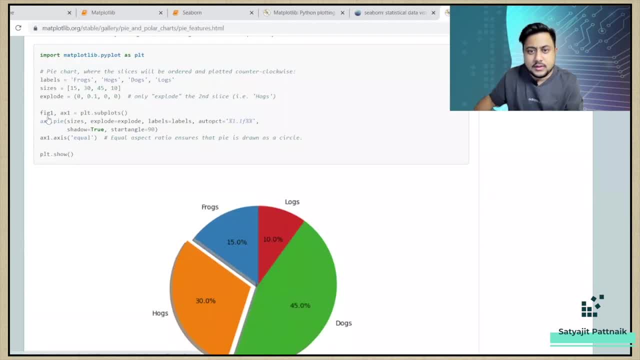 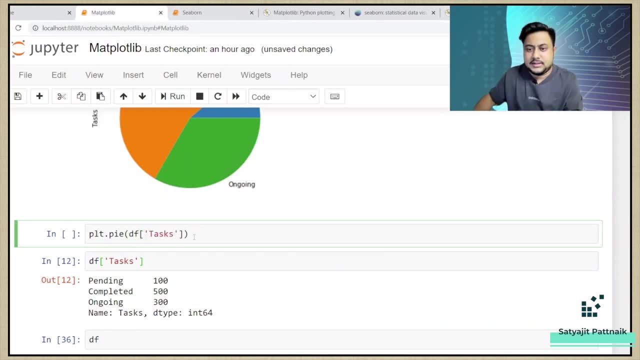 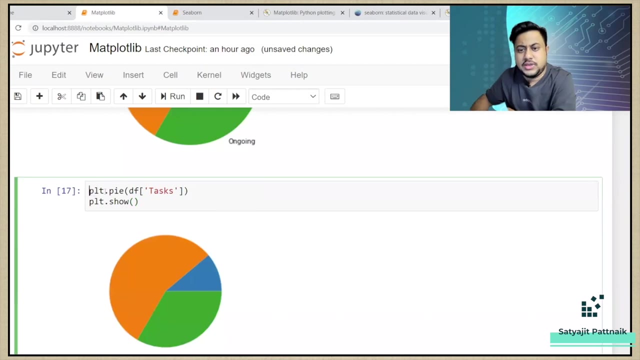 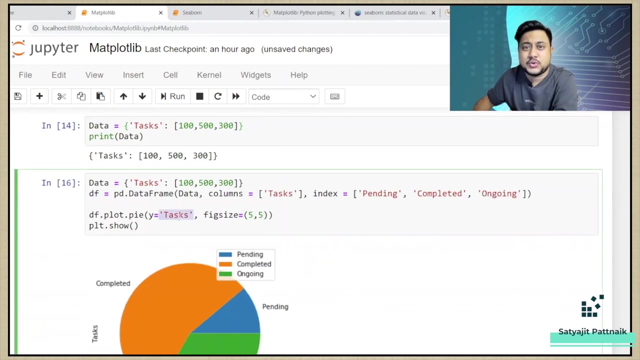 pltpi. okay, okay, so let's just call this df of tasks and then i will just do randomly. i'm just doing something and let's see, you can see, same thing has also been created. so here i am able to pass the data frame column tasks, but here the, if i pass y equals to df of this. it will fail because 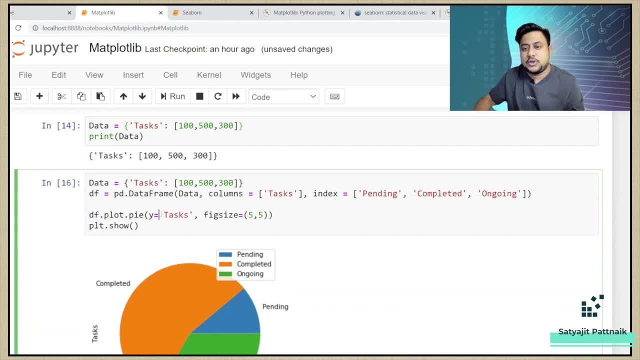 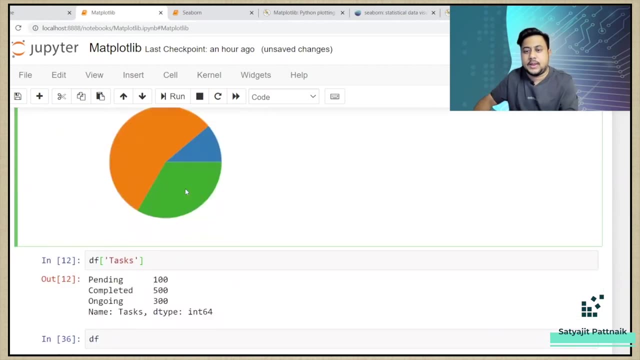 here i'm calling the pandas data frame itself, right, so? so just you have to pass tasks column because it already knows this data frame. so either you can create a chart using the pandas library or else using the matplotlib. so this is how you create a matplotlib library. okay, 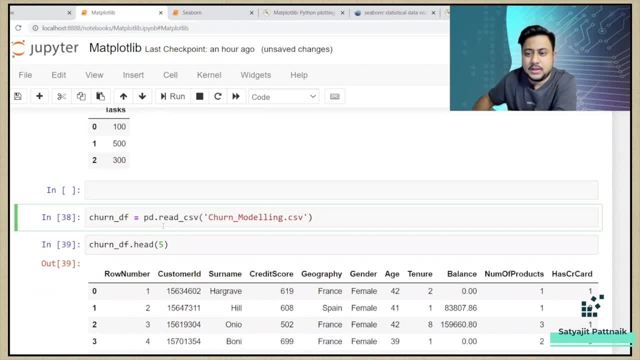 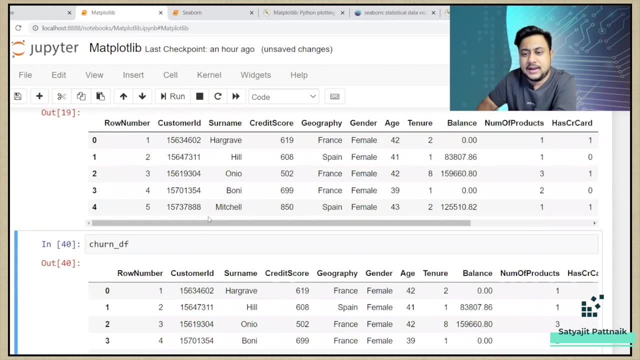 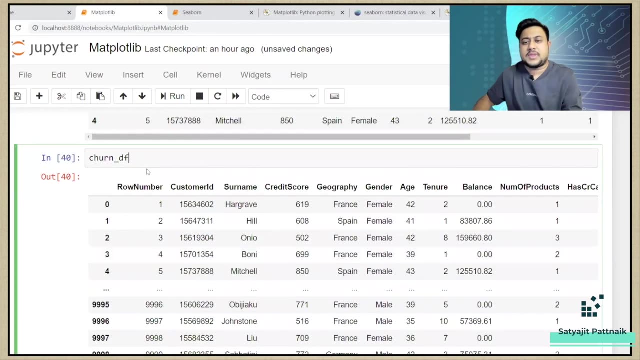 and then what else? here we are reading a file, so the same file which we had done using pandas, churn, underscore modeling. if i have to run this dot head, this is how my data set looks like. and let's say, i have my y variable, which is my exited. now how to see the 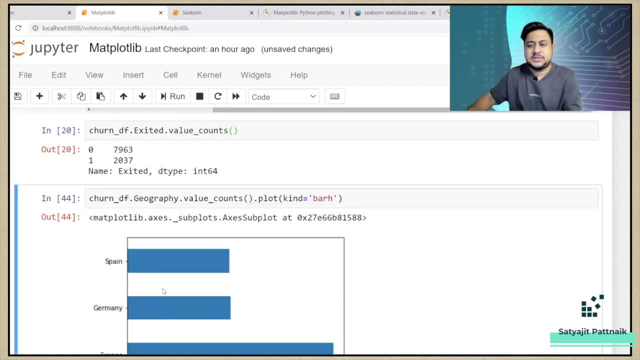 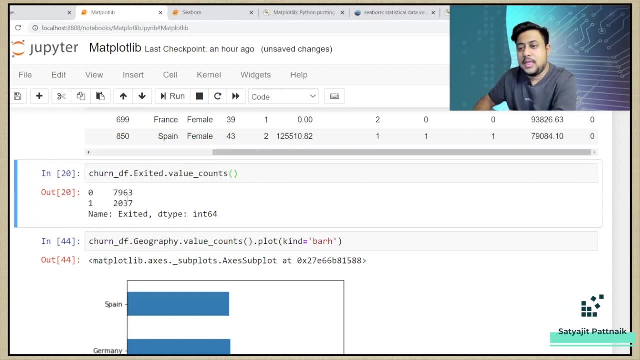 value counts of this column value counts is basically giving me: i have 7 900 records for class 0 and 2000 records for class 1.. how to create a bar chart out of it? it's pretty simple: dot plot kind equals to bar. if you just do this, a bar chart will be created. 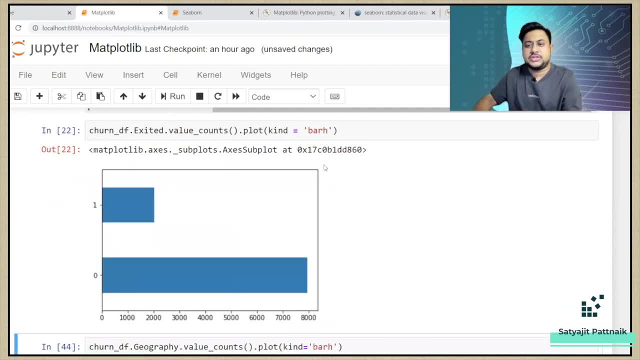 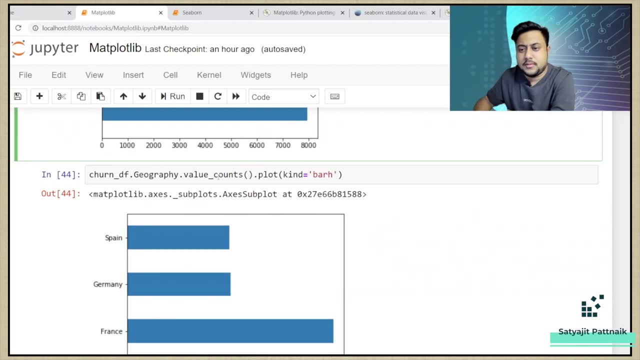 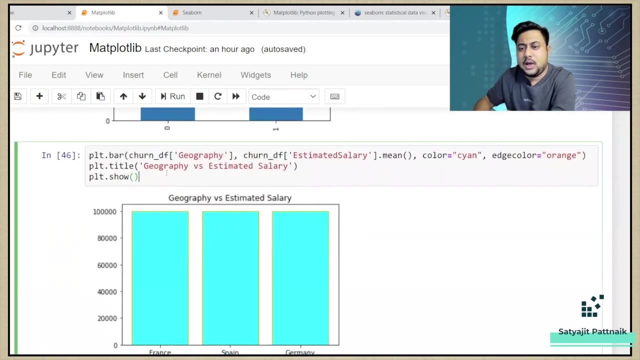 if you want a horizontal bar chart, you can do bar h. so this is how you can also plot a bar chart using value counts dot plot. okay, apart from that, again same things. plot kind equals to bar. now, here we are not doing anything extra, we are just calling plot dot bar. that means matplotlib dot bar. 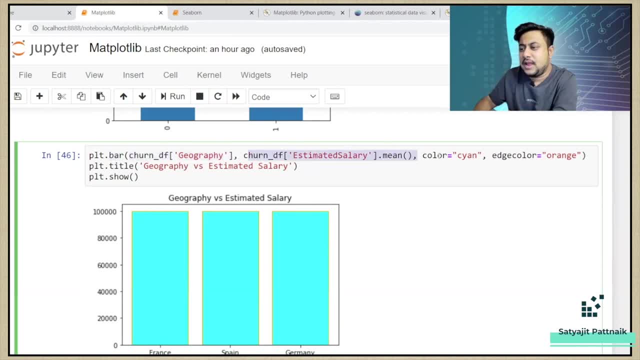 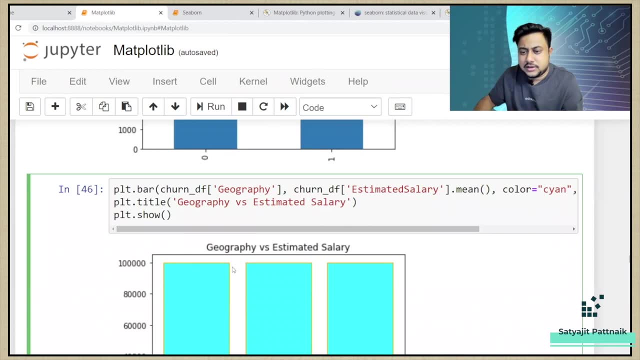 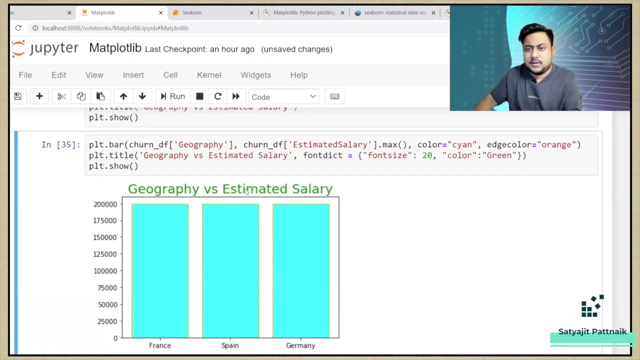 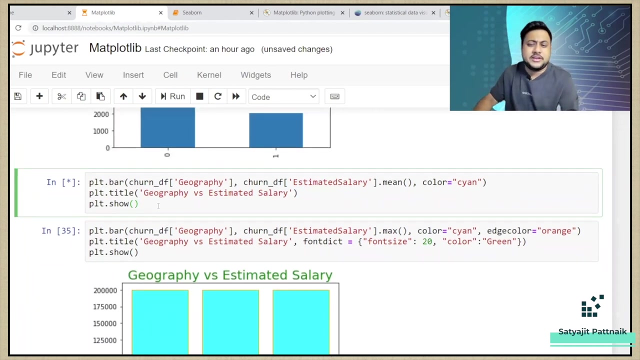 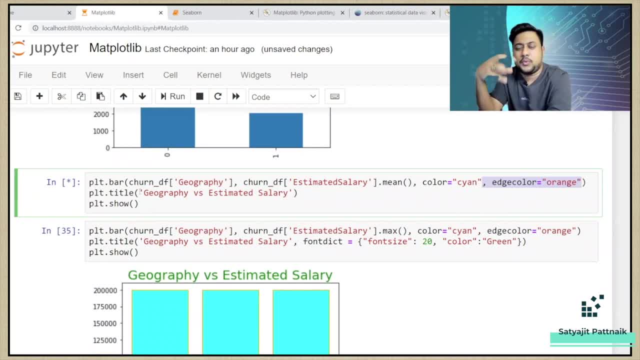 provide a title to your graph. okay, if you want to add labelings on x axis and on y axis, there are methods called as plt dot x label and plt dot y label. i'm not pretty sure why it's taking so much of time, but you can see same piece of code. let it finish. we'll jump on to the next one. so 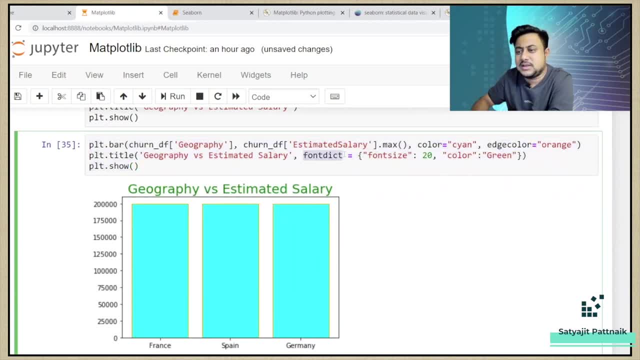 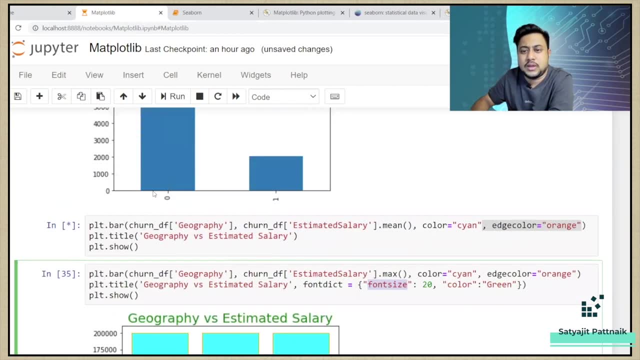 here we have the same piece of code, but here i'm passing a font dictionary where i'm passing the font size as this and color equals to green. this is my title. okay, it should have already run by this time. not pretty sure why it's not running. okay, let's move on to the next ones again here. 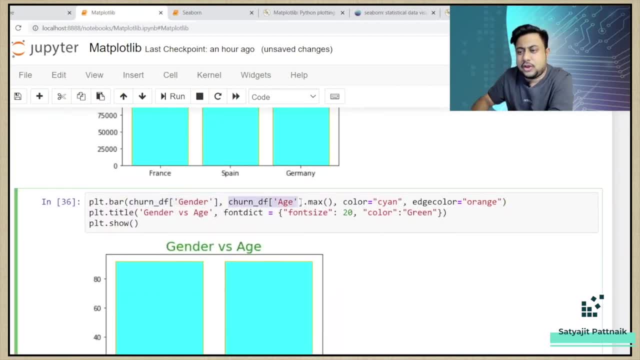 i have done the same thing, column a, column b, dot max, and then i have passed some color which is my cyan and my edge color which is my orange. here i'm before your show method. i'm just calling the dot title which basically is telling me gender versus age. here my font dictionary is: 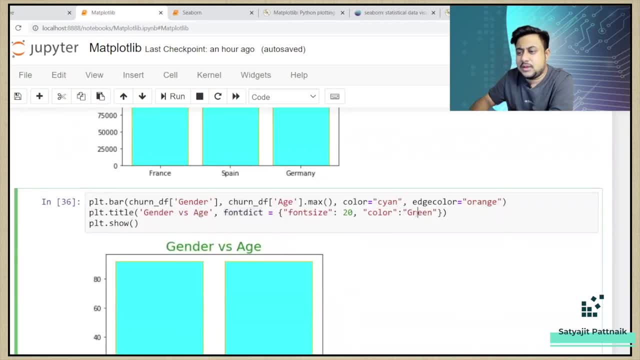 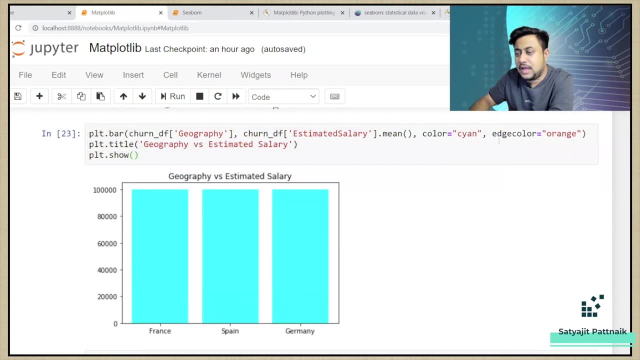 20. here you can see, i think everything is same color equals to green. that's it. oh, that this has run. you can see, here there is orange and here i have just ignored- i had ignored it right while i run this, i had ignored this- so there is no edge color. so if you provide edge color as blue orange, 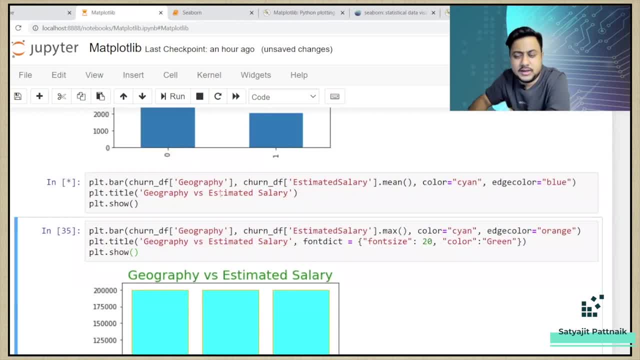 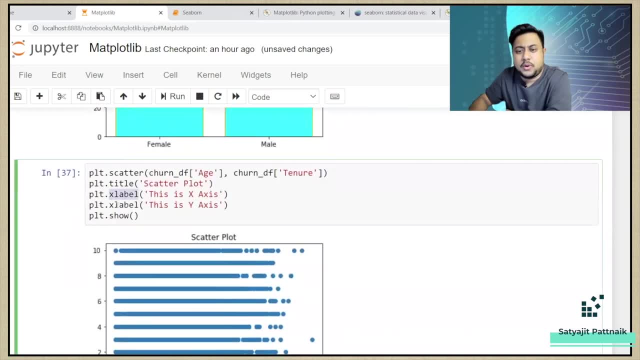 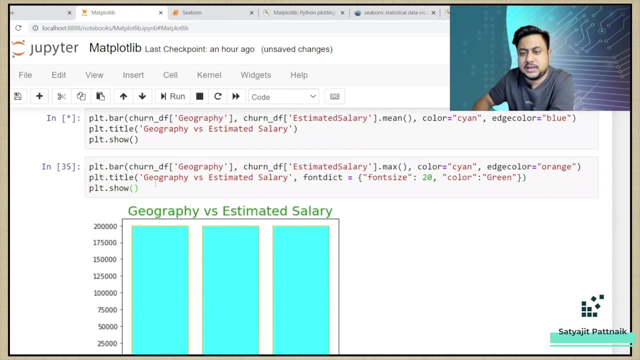 all these things, and that's that's how it will work. right, it is taking a little bit time. let's jump onto the next ones. yes, i already told about x label and y label. this is how you're okay, so my first code is already running, so that's the reason it will take a little bit of time, but you can see. 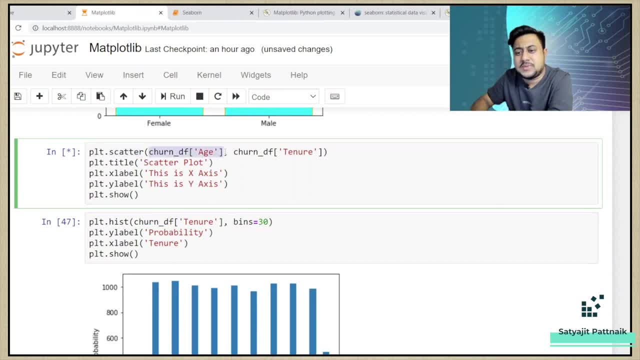 this code: plt dot- scatter. i have passed my x, my y, and then i'm calling my title, which is my title of the graph, my x label, my y label, and then plt dot show here same thing, same piece of code, instead of scatter. i'm just doing this, trust me, guys. you. 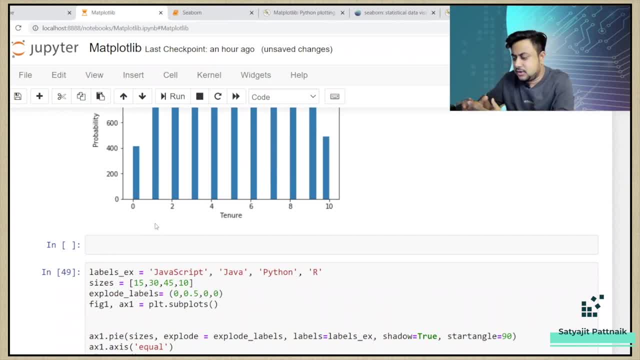 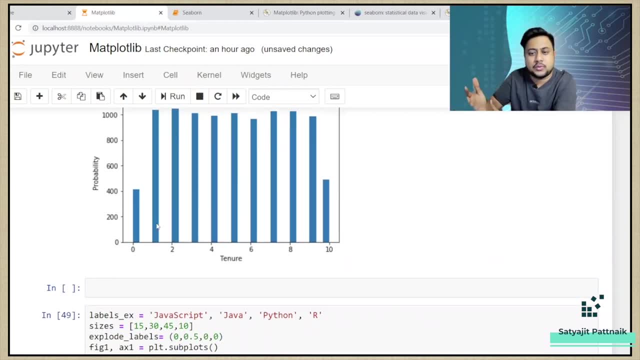 just have to explore, like if in case tomorrow you want to create some histograms, you don't have to memorize all these things, you have the community. simply just google it out. you will find the codes and just copy paste it. work on it, practice, practice, practice and then definitely you will. 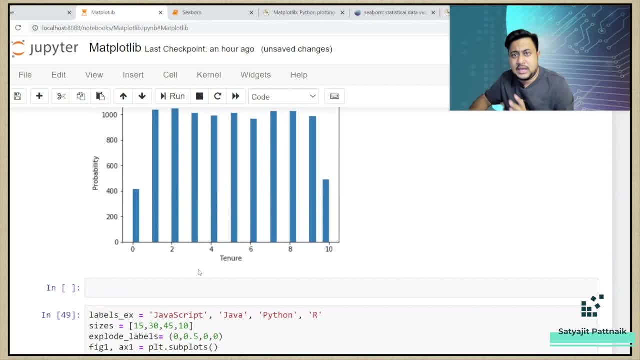 succeed right, trust me, many of the codes. even i am not pretty aware of that, even today's data, so i search in the google. whenever i have to plot, i have to do a search on that. so, yes, everything has been done. you can see edge color equals to blue and this is how it looks like. 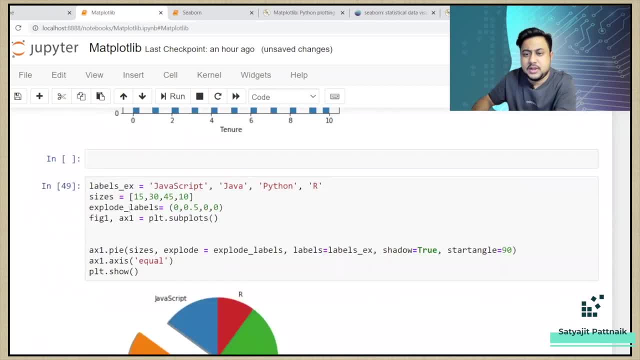 right, jumping back to the last part, which is exploding what? what is basically a pie chart? exploding, that means i want to have an explosion of one of the parameters. now here i have javascript, i have java, i have python, i have java, i have java, i have python. i have python, i have python, i have. 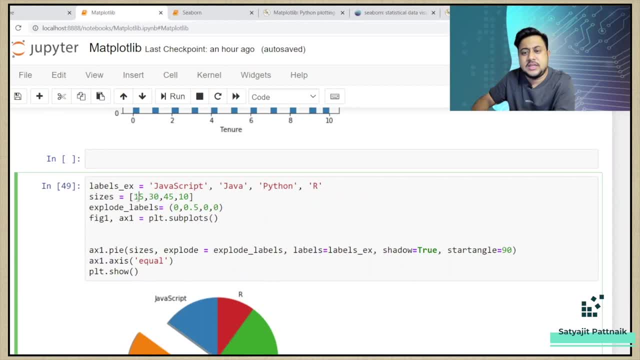 have our sizes. I have 1530. that means 15%, 30%, 45%, 10%. explode levels is 00.500.. That means I want my second item to explode from the graph, the Java to explode from the ground. 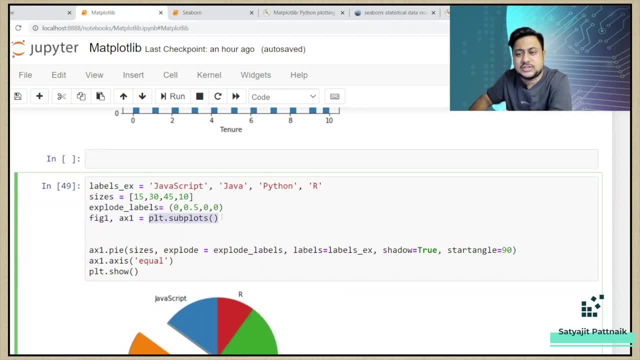 So here I'm calling figure one: x one PLT dot subplots. So in case you are creating multiple plots within a plot, then you have to call subplots. here again, x one dot pi. I have just defined sizes. explode equals to explode level, just in case you don't know about explode. 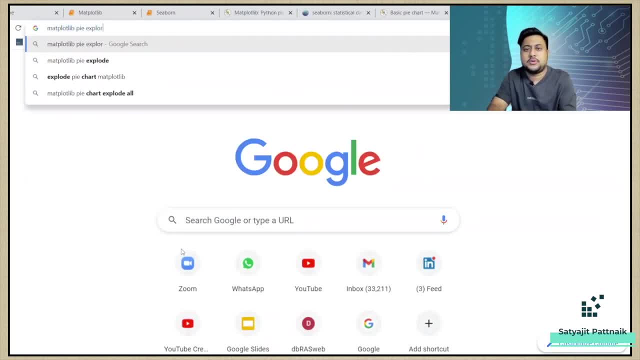 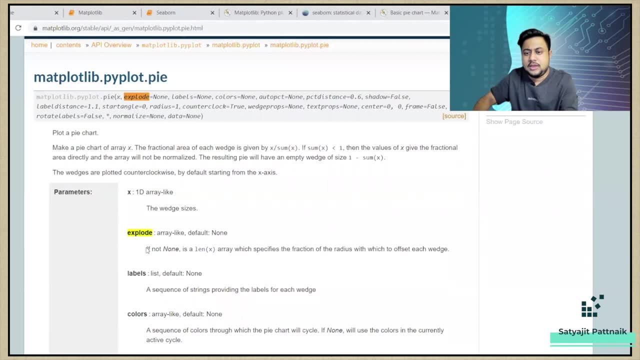 simply matplotlib pi: explode Everything. the community is so great, you just have to search it and you will understand. explode If not. none is a length of array which specifies the fraction of the radius with which To offset each wedge. that means each wedge or each division has to be separated out. 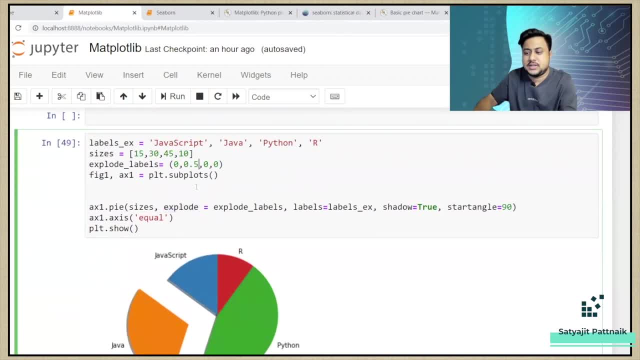 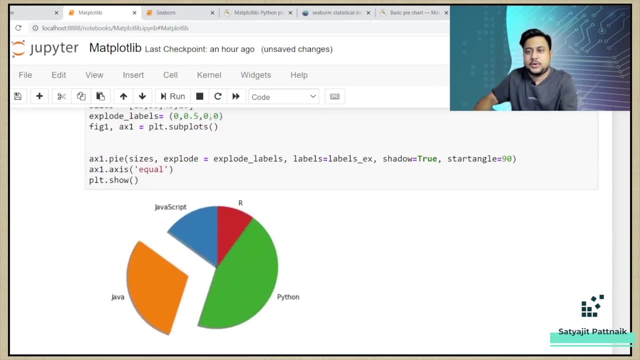 it has to be exploded. If I just pass 0.1, run it. This is how it looks like. if it, if it is 0.5.. This is how it looks like. If you want to provide another explosion, then this. 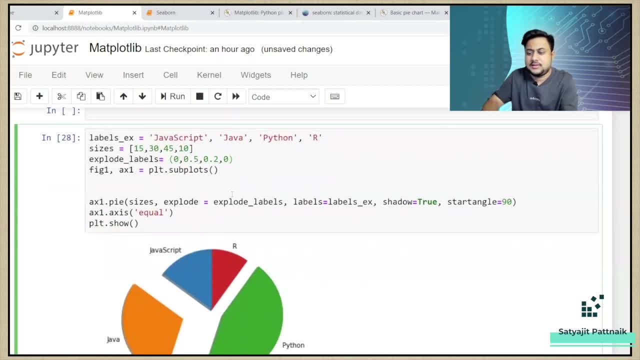 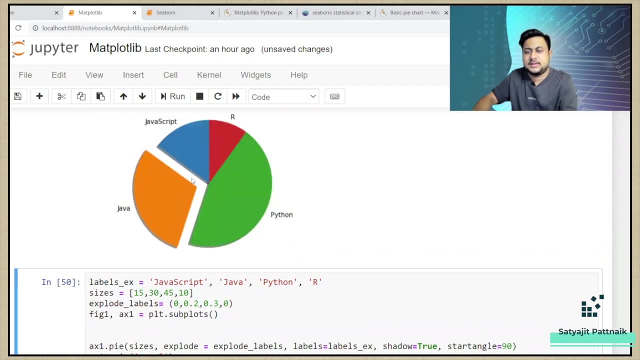 is how it looks: like Python has been exploded, Right, And this is how things works. Okay, I'm just reverting back. Let's say point two, I think, I think. And then this is how you can do your explode explosions, Okay, And then how? 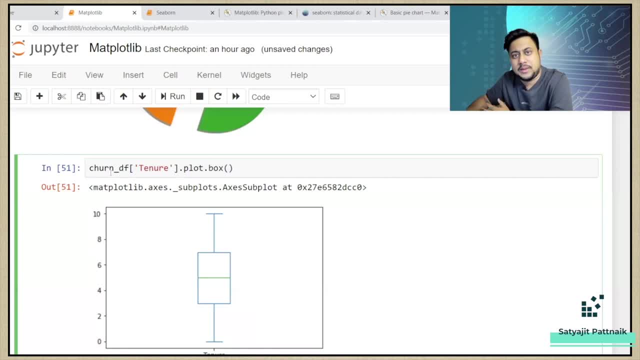 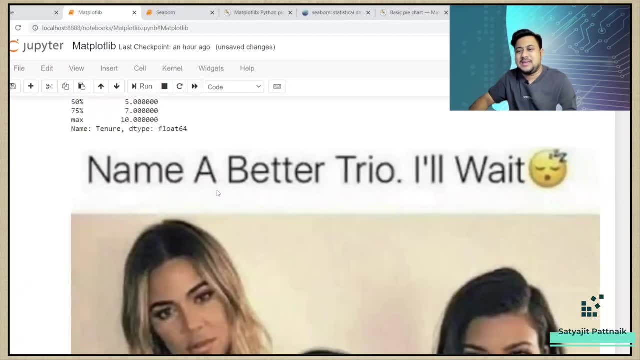 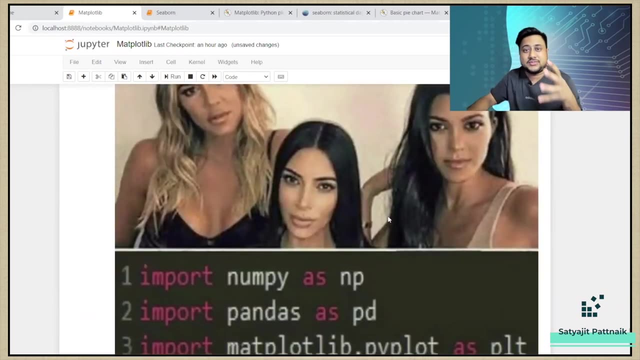 to create a box plot again. data frame, column name: dot plot, dot box. Okay, So this is just a small meme name, a better trial, I will wait. So the way to try to raise numpy pandas and matplotlib, because these are the three things which any data scientist writes before doing. 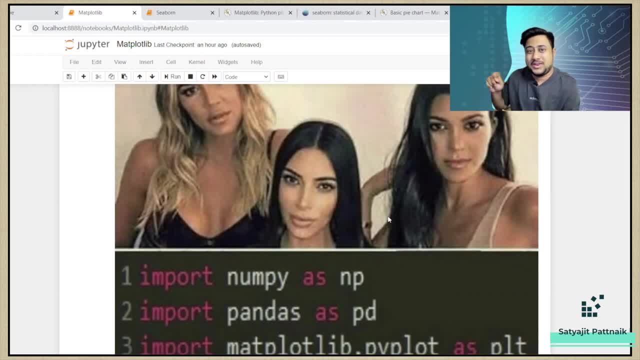 any piece of code It's like: Okay, I can do this, Let me do this, Let me do this. Let's like, if you are a Hindu, we write Ong or Sriganesh, something like that in examination papers. 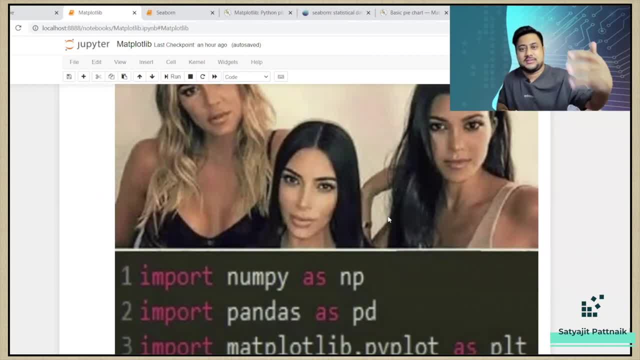 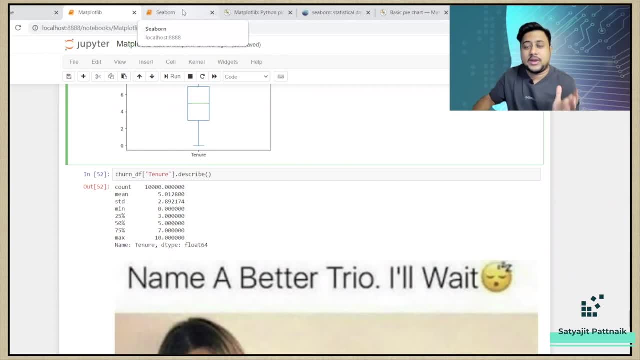 And this is something like that. It has to be starting with these three lines. So that's it from my side, guys. And well, oh my god, how can I forget? I have Seaborn to cover as well. So let's start with Seaborn. 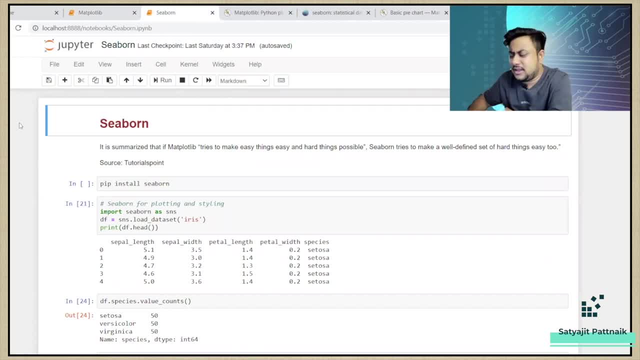 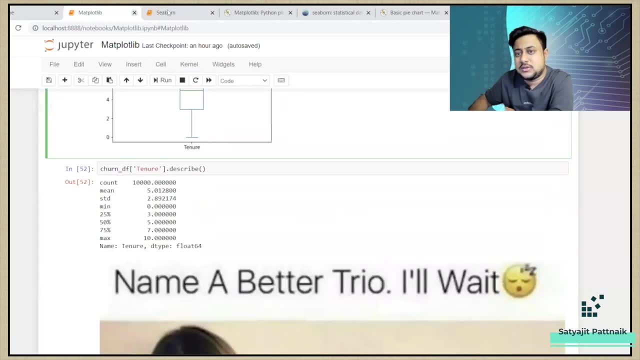 Again: Seaborn, Matplotlib, Dash. there are many, many such libraries. If you just focus on libraries, you will not succeed, probably. So, just randomly, you can do any of this. If you are just plotting it, just plot any of them. 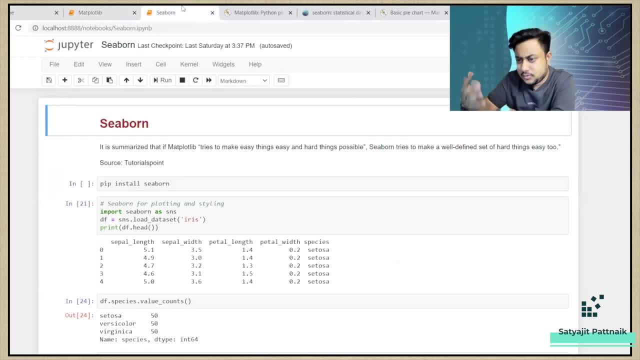 Because ultimately, the plots which you will be using in your code, this is just for you, This is just for a developer right, Because you cannot show that plots to your manager or to somebody else, Because for that you will have to create. 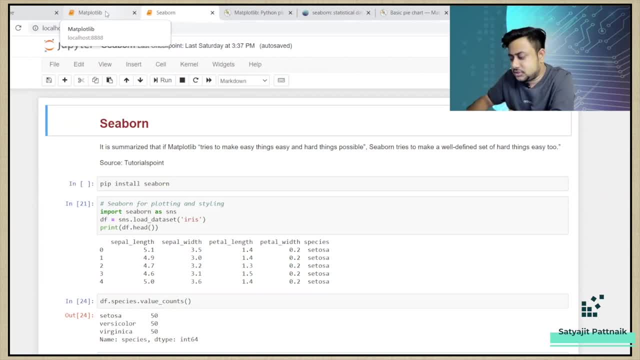 really good visualizations, So for that you might need presentations, PPTs, Excel, Power BI or anything else. So if you are just doing on Python, Matplotlib, Seaborn doesn't really matter, You can do anything. 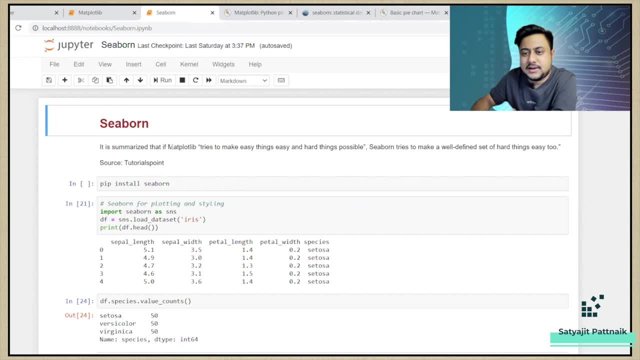 It's just another library, right? So it is summarized that if Matplotlib tries to make easy things easy and hard things possible, Seaborn tries to make a well-defined set of hard things easy too. I mean, yes, Seaborn is a little bit easier. 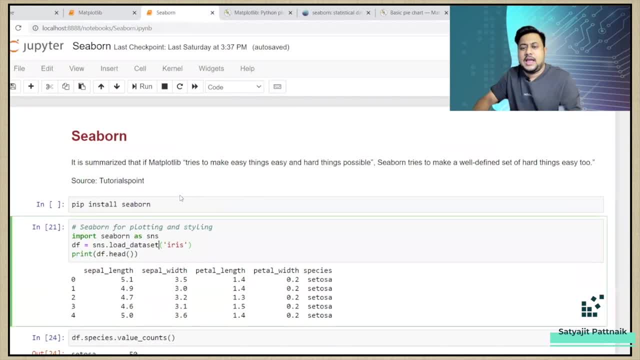 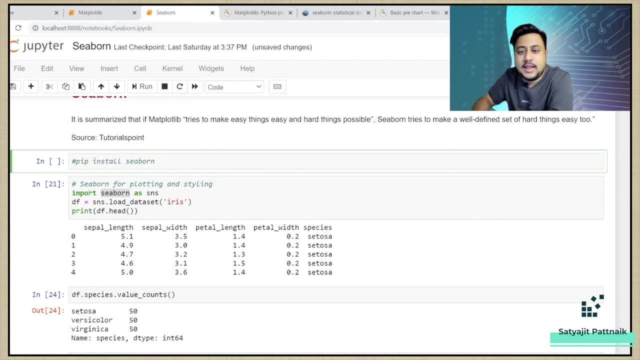 as compared to Matplotlib. So here I am importing Seaborn. In case you don't have Seaborn, you just have to install it using pip install- I'm just commenting it out And then importing Seaborn as SNS. 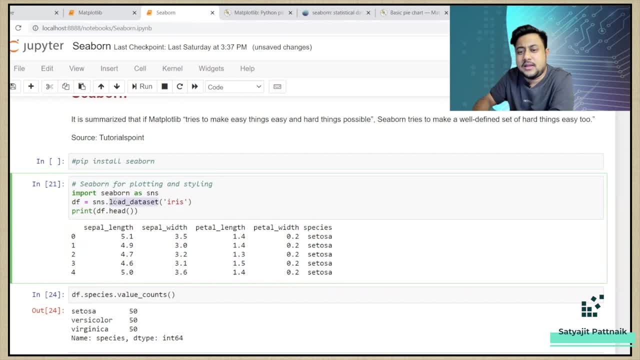 SNS is my alias. Here I'm loading a data set, So in between, by default, many such libraries are there, which already has some predefined data sets, like Iris data set- Iris data set is very common, Iris, Penguin- many such data sets. 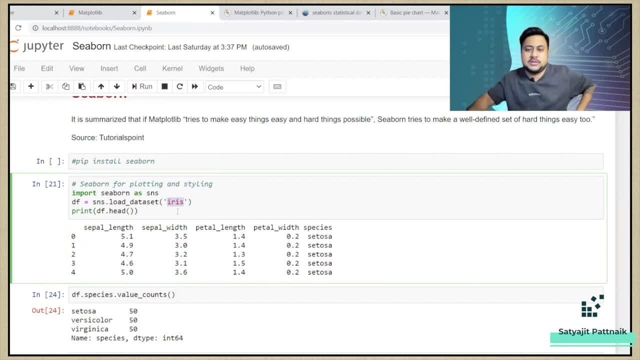 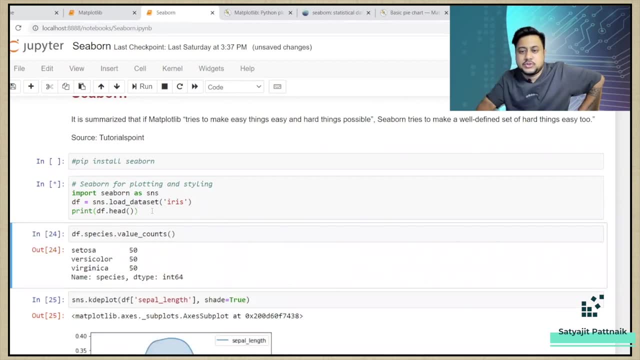 are there which are actually preloaded in those libraries. So Seaborn has a lot of libraries, a lot of data sets, out of which Iris is one of them. So if I just do this, that means it's fetching the data from the Iris and then going dfhead. 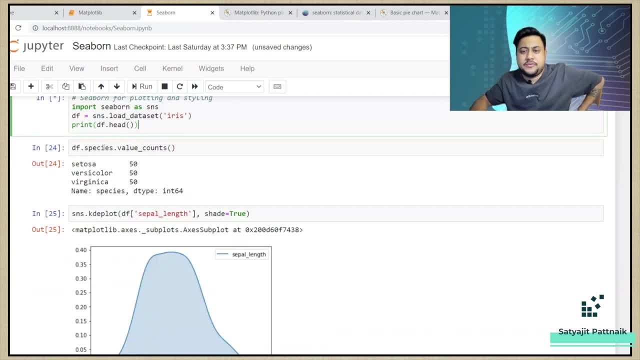 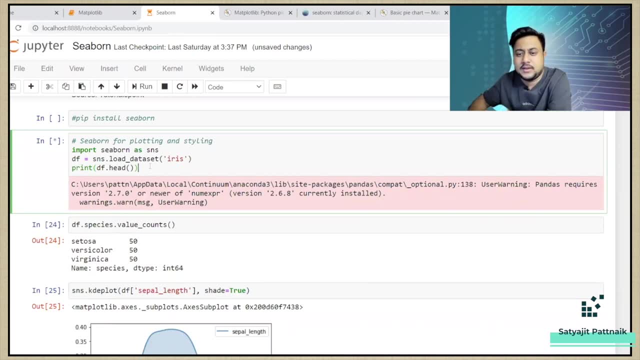 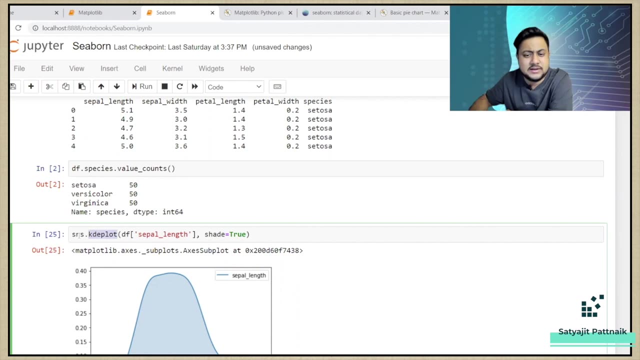 So let it finish. And then I have speciesvalueCount. So species is nothing but my y variable, right? So I'm just doing my value counts here And then I'm calling the KDE plot. As simple as that. SNS is going to be very simple. Seabornplot. 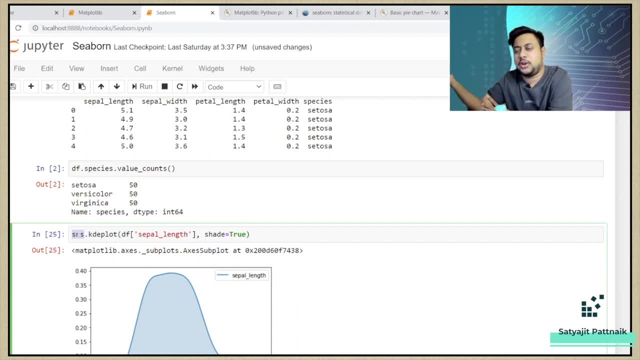 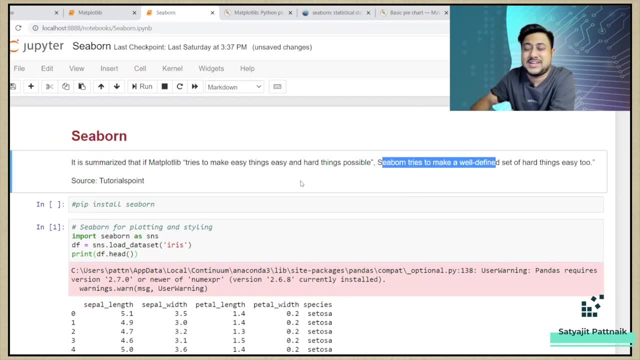 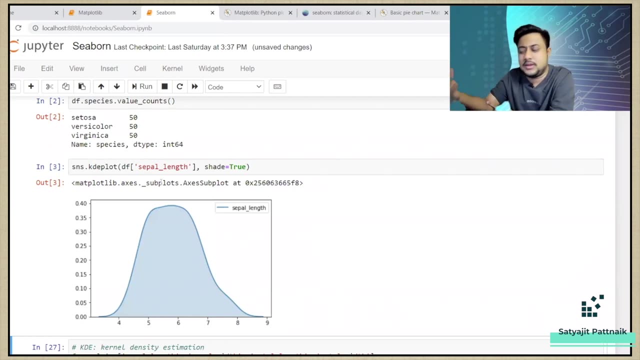 That's it, And then inside your plot you just pass your columns. That's how simple Seaborn is. That's the reason it is told that Seaborn tries to make a well-defined set of hard things easy too. So KDE plots is nothing but a kernel density estimation plot. 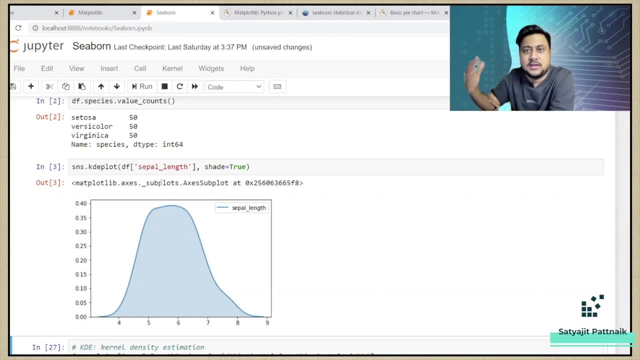 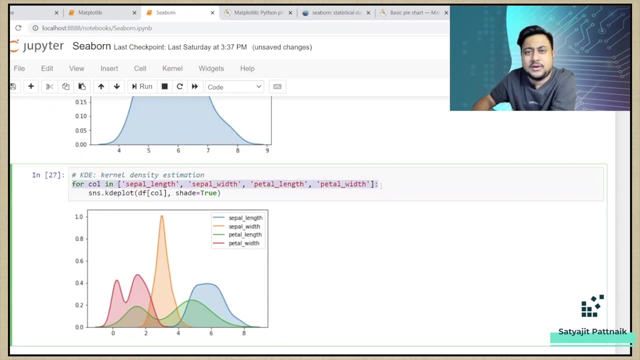 It's just it gives you a density distribution kind of thing. OK, If you are keen to learn about what exactly is KDE plot, go to Google Dev, right, And then here, what I'm doing is I'm just running for a loop of different columns. 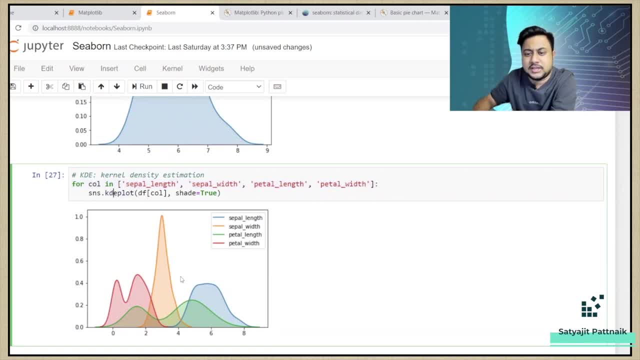 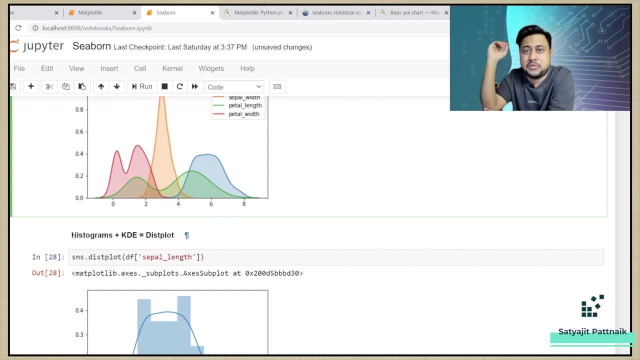 and then I'm plotting it. So I'm just plotting different graphs, the different kernel density graphs. OK, Histograms plus KDE will basically give you a distplot, right. So snsdistplot, column name: Very simple. Seaborn is going to be very simple. 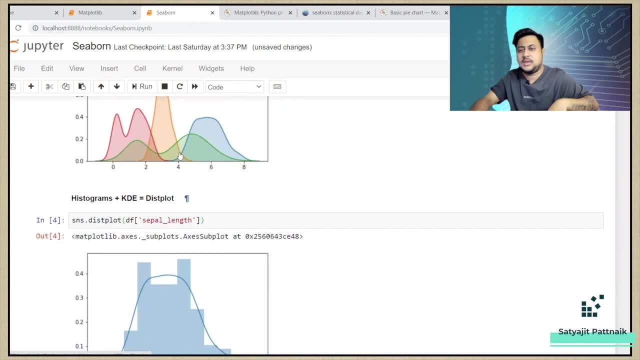 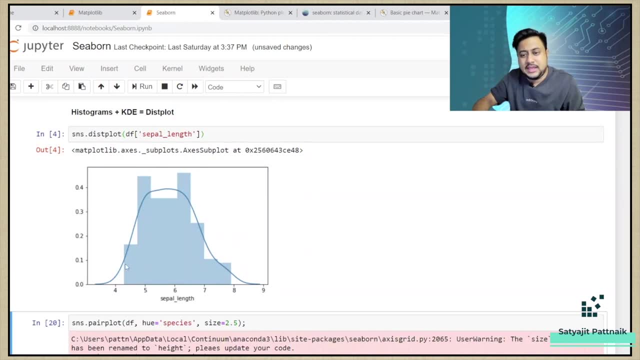 For you. that's the reason I have just kept two or three plots, And the rest of them you can just explore by yourself, And then you can see it's a combination of a KDE, which is this line, And then you can also see some histograms, right. 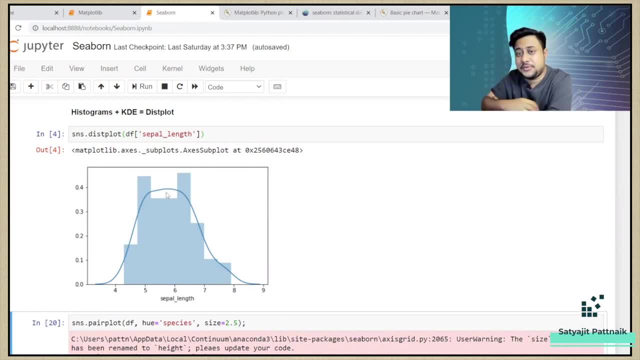 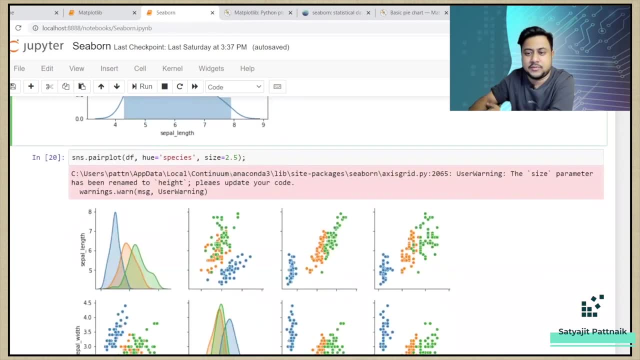 So how to interpret and all those things. I'll probably have a video on that, But this video is especially for the different methods inside your Seaborn and Matplotlib. I was talking about pair plot. right, If you have 10 variables, it's going. 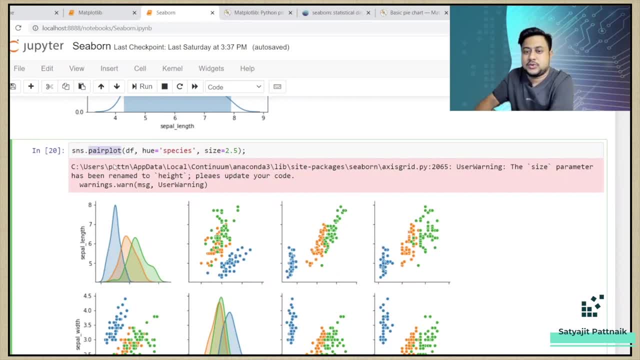 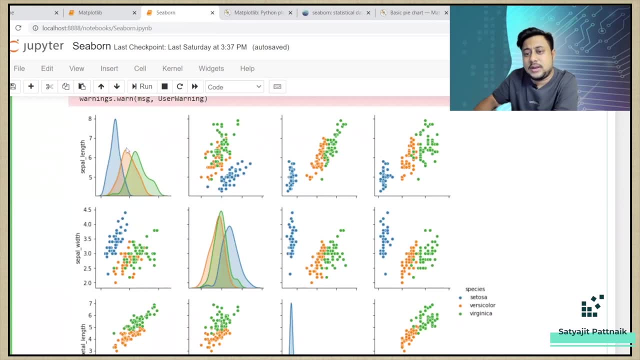 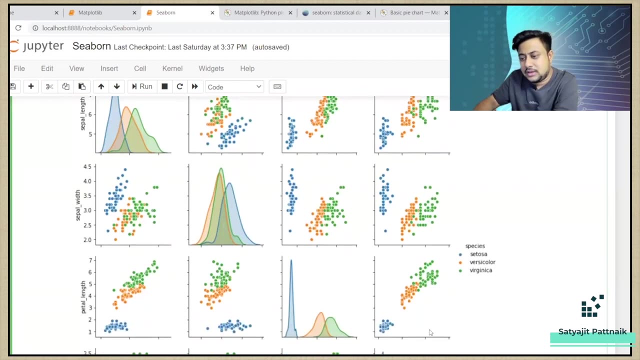 to be a 10 cross 10 visualization matrix. So here we have four variables. So that's the reason It's basically 4 cross 4.. How to see or how to interpret a pair plot? Just ignore the diagonals. Let's say you will talk about this particular graph. 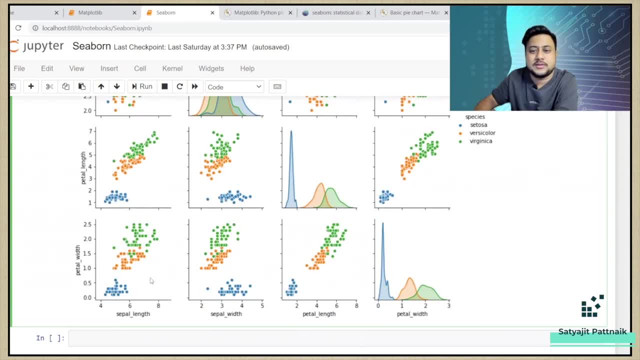 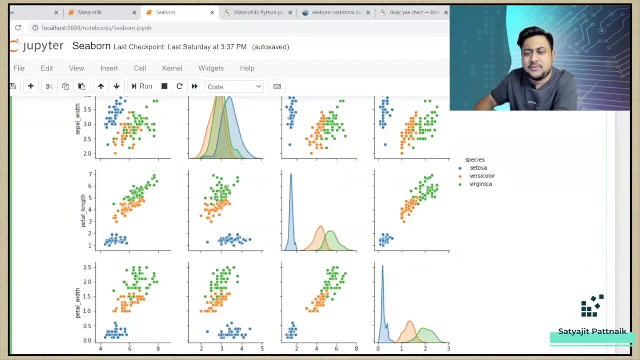 This means petal length versus sepal length. So for this class for blue class, which is setosa for setosa, I don't see a very good linear relationship. That means, if my sepal length is increasing, my petal length is not increasing.